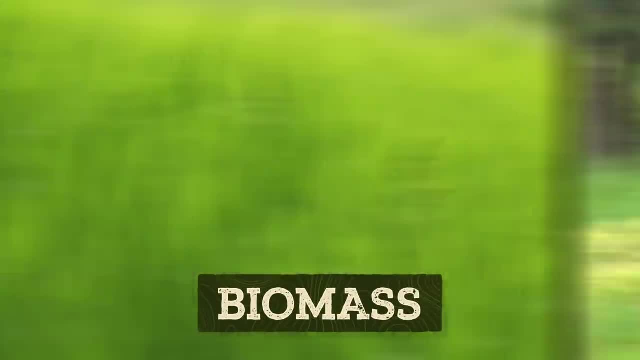 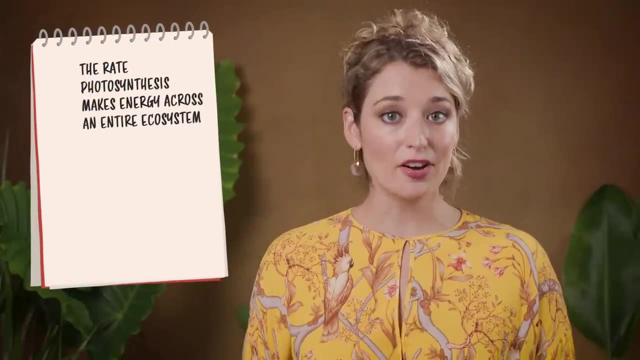 which is stored in biomass, any plant or other living thing. If a bit of biomass is eaten, it passes on its chemical energy to continue the energy flow. The rate photosynthesis makes energy across an entire ecosystem, minus the rate that energy is used, is its net primary production. 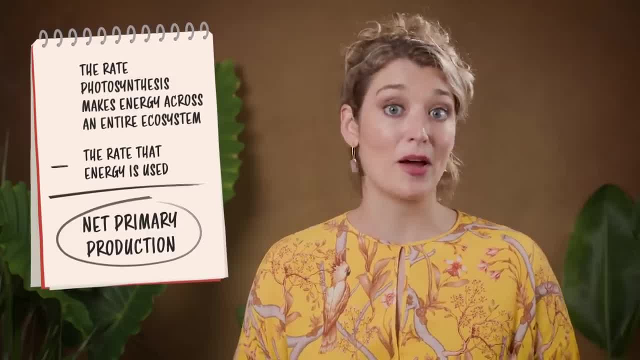 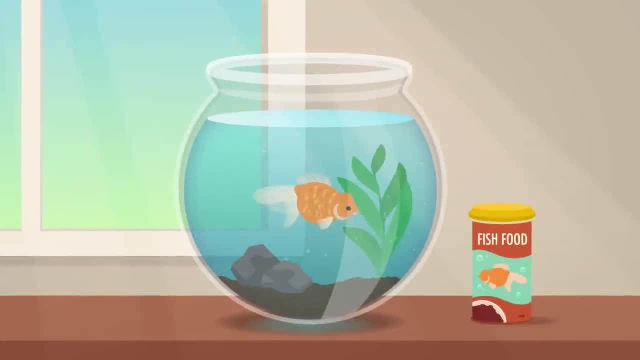 or the amount of stored chemical energy in an ecosystem over a certain amount of time, For example, on a really small scale. think of a fish tank ecosystem that you can hold in your hands. There's water, a fish, soil, rocks, air, light, food and one little plant, all in a glass bowl. 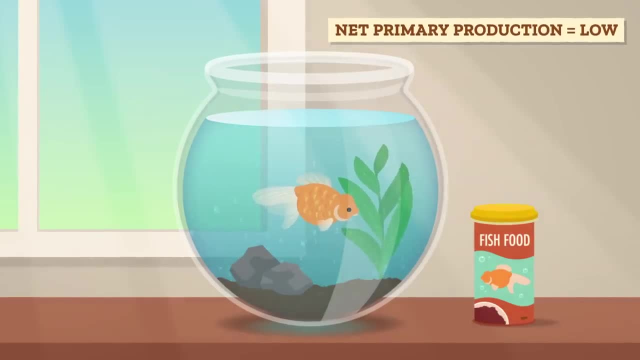 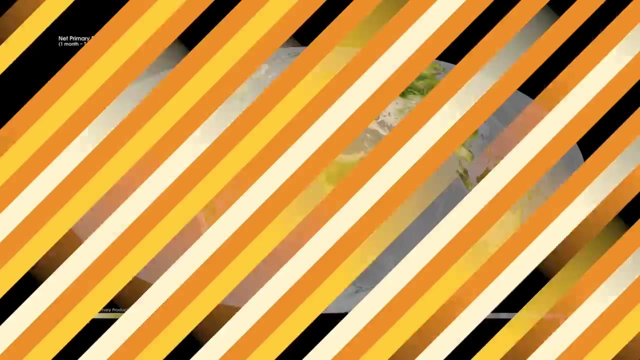 In this fish tank ecosystem, the net primary production is pretty low because only that one little plant is absorbing energy from the sun, along with any photosynthetic bacteria or algae that grows when I forget to clean the bowl. Globally, net primary production on land generally changes with latitude. 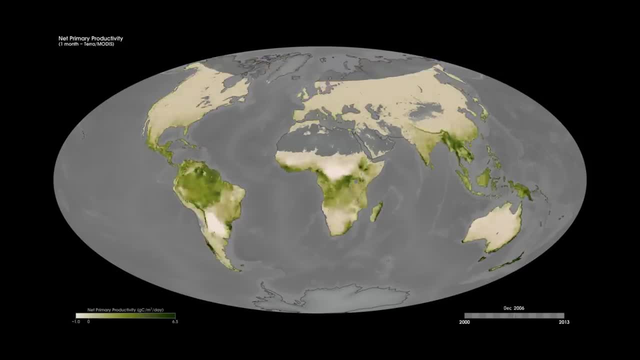 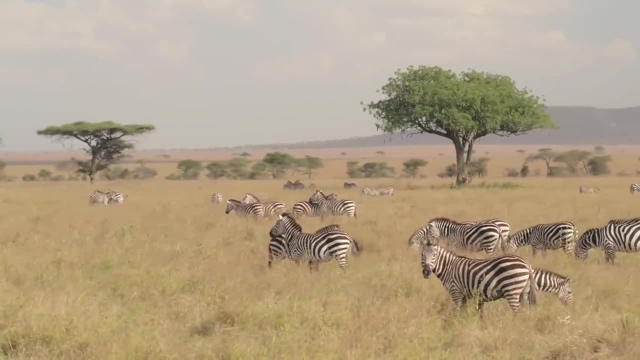 Productivity is highest between the tropics and decreases towards higher latitudes and elevations. Biogeographers and ecologists who study how life is distributed on Earth probably figured that calling regions of the world a very productive ecosystem or extremely not productive ecosystem would be pretty boring. 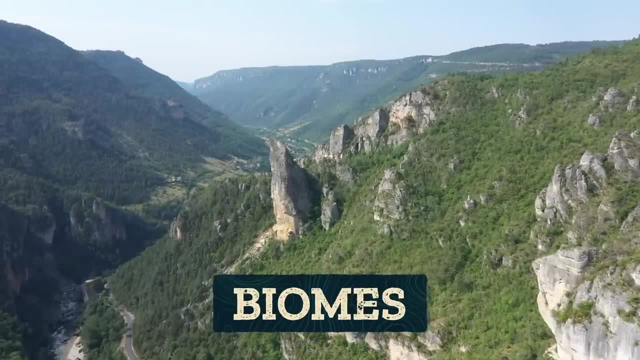 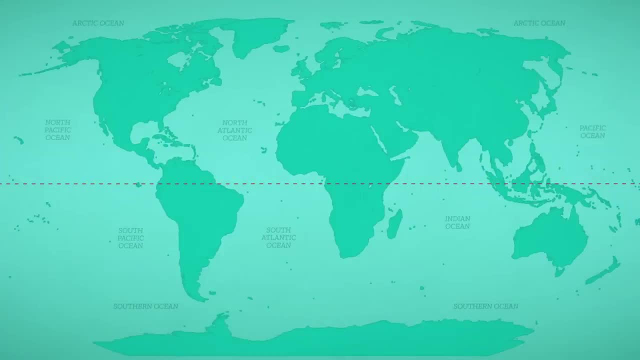 Instead, we classify ecosystems into biomes or habitats with similar characteristics, including productivity. The names are much more descriptive and fun. The equator gets the most sunlight and a lot of precipitation, so there's a lot of photosynthesis happening here. 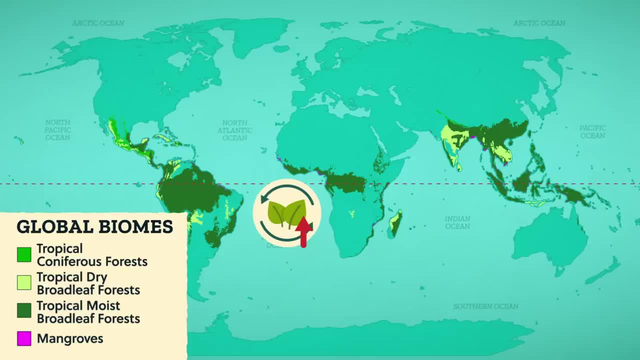 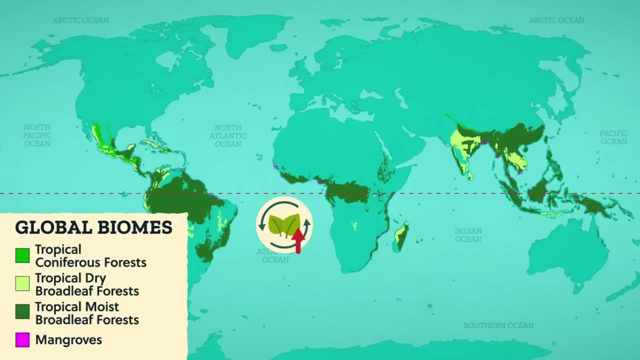 These highly productive ecosystems are all tropical rainforest biomes, which are some of the most diverse and complex areas of the planet, So it's no wonder the tear-drinking moth lives here. Similar patterns happen on either side of the equator, but we're going to turn north because there's more land in the northern hemisphere. 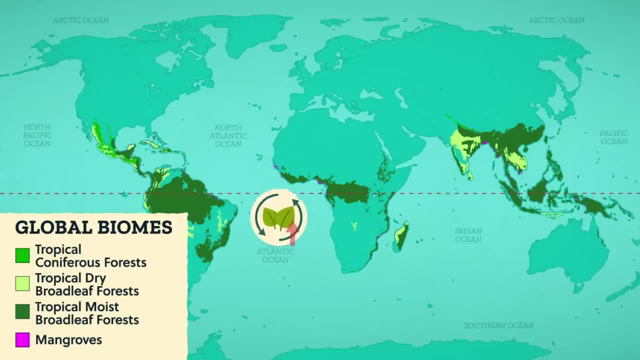 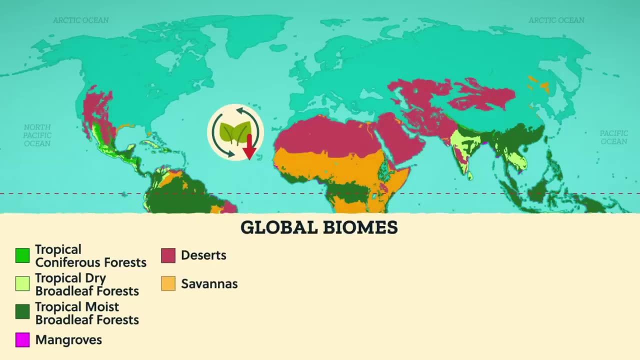 There's also less and less precipitation as we move out from the equator and less and less productivity, because photosynthesis can't happen without water. The biomes gradually shift from tropical rainforests to tropical savannah, to desert Further north, in temperate and high latitudes. the net primary production varies seasonally. 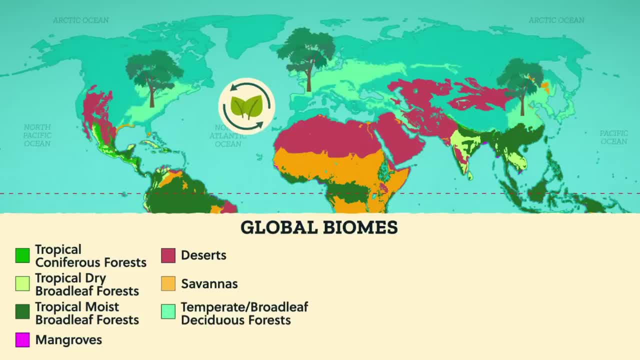 Like one biome, is the broadleaf deciduous forest with oak, beech, hickory, maple, elm and chestnut. These trees have increased productivity in the sunny spring and summer and shed their leaves in the cooler fall and winter seasons. 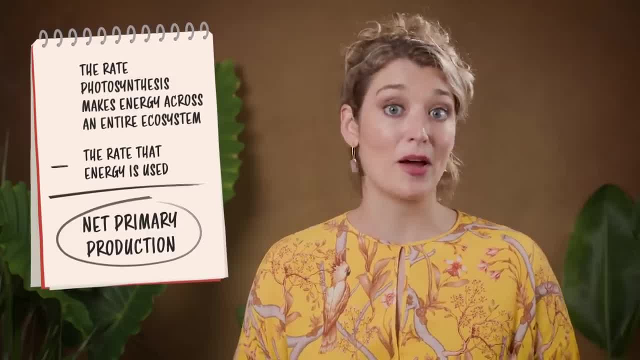 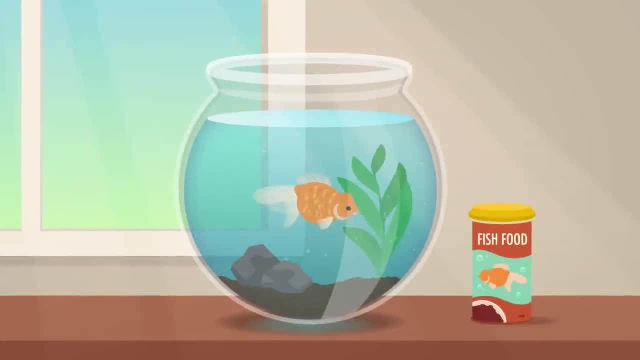 or the amount of stored chemical energy in an ecosystem over a certain amount of time, For example, on a really small scale. think of a fish tank ecosystem that you can hold in your hands. There's water, a fish, soil, rocks, air, light, food and one little plant, all in a glass bowl. 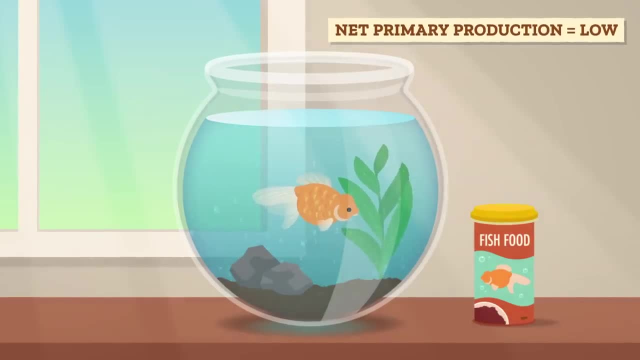 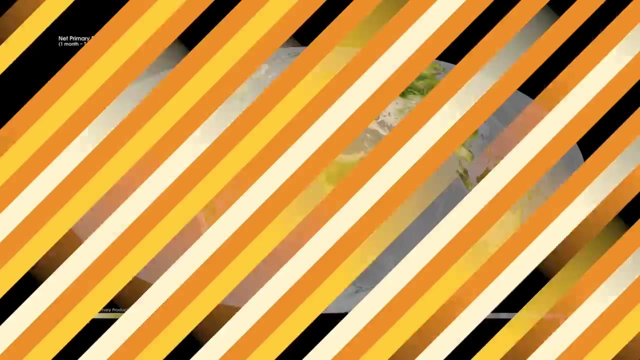 In this fish tank ecosystem, the net primary production is pretty low because only that one little plant is absorbing energy from the sun, along with any photosynthetic bacteria or algae that grows when I forget to clean the bowl. Globally, net primary production on land generally changes with latitude. 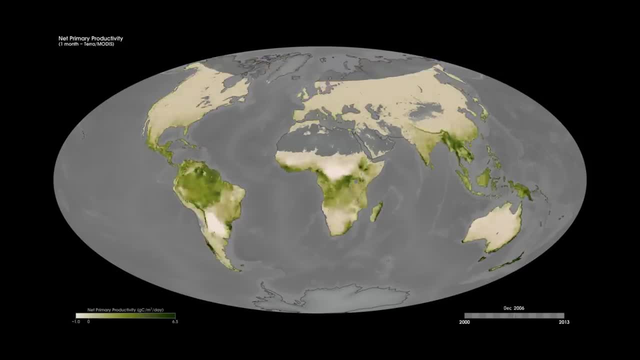 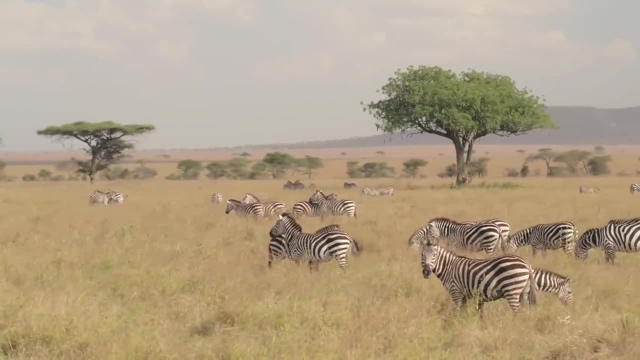 Productivity is highest between the tropics and decreases towards higher latitudes and elevations. Biogeographers and ecologists who study how life is distributed on Earth probably figured that calling regions of the world a very productive ecosystem or extremely not productive ecosystem would be pretty boring. 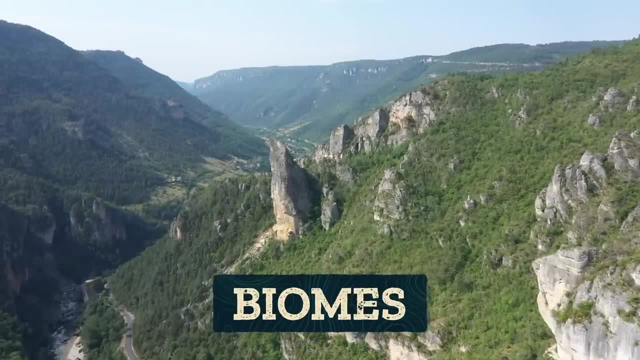 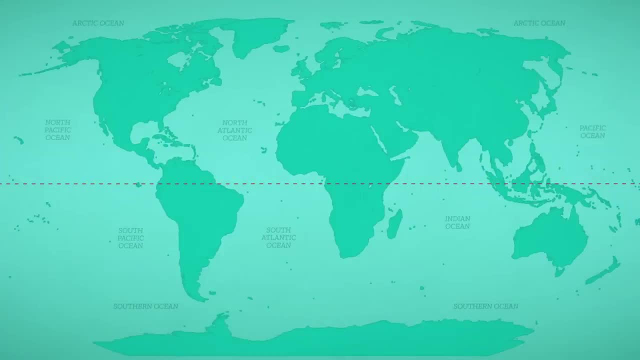 Instead, we classify ecosystems into biomes or habitats with similar characteristics, including productivity. The names are much more descriptive and fun. The equator gets the most sunlight and a lot of precipitation, so there's a lot of photosynthesis happening here. 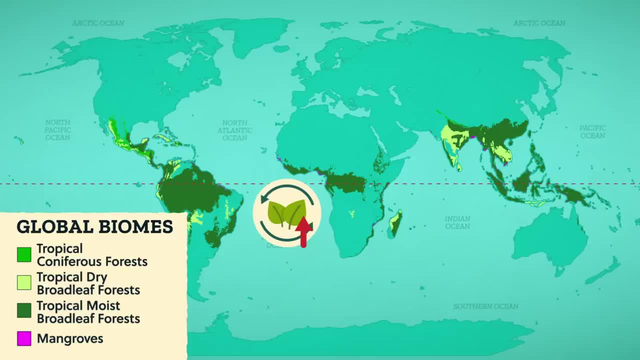 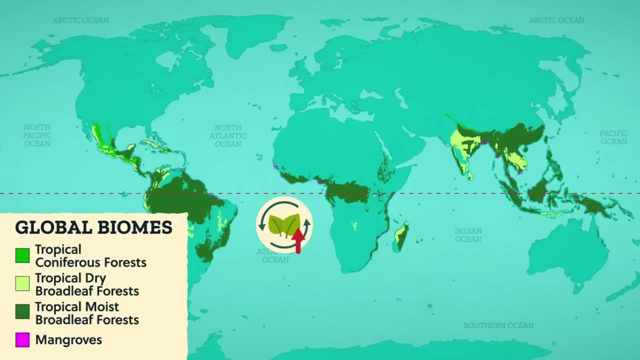 These highly productive ecosystems are all tropical rainforest biomes, which are some of the most diverse and complex areas of the planet, So it's no wonder the tear-drinking moth lives here. Similar patterns happen on either side of the equator, but we're going to turn north because there's more land in the northern hemisphere. 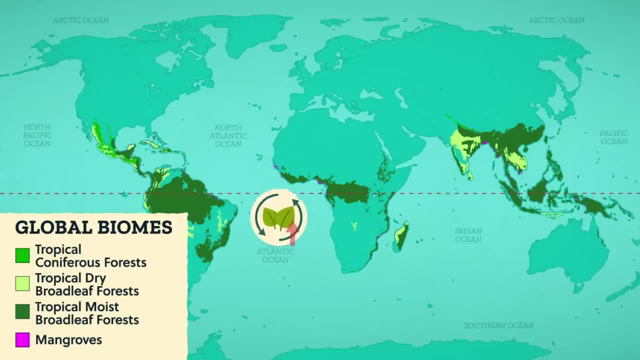 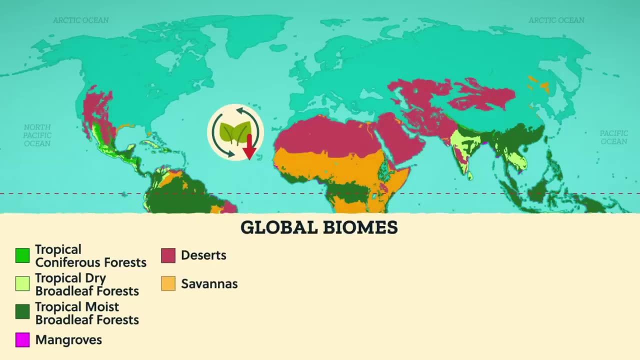 There's also less and less precipitation as we move out from the equator and less and less productivity, because photosynthesis can't happen without water. The biomes gradually shift from tropical rainforests to tropical savannah, to desert Further north, in temperate and high latitudes. the net primary production varies seasonally. 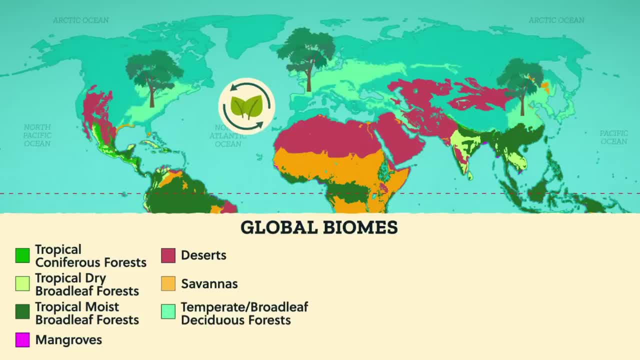 Like one biome, is the broadleaf deciduous forest with oak, beech, hickory, maple, elm and chestnut. These trees have increased productivity in the sunny spring and summer and shed their leaves in the cooler fall and winter seasons. 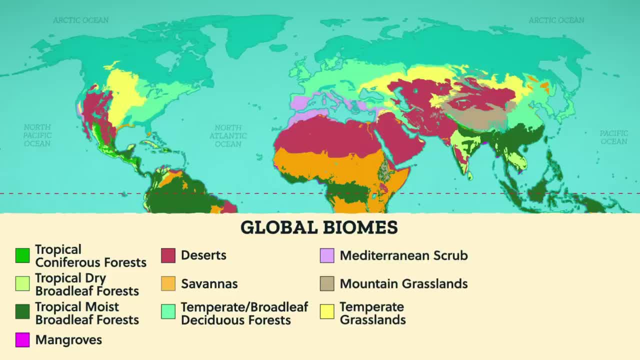 Up here in the middle of continents, there are temperate grassland biomes with rich soils that produce the tall grass of prairies and the short grass of steppe climates. Further north, where there are poorer soils and colder climates, we meet the boreal forest biomes, which have mainly evergreen pine. 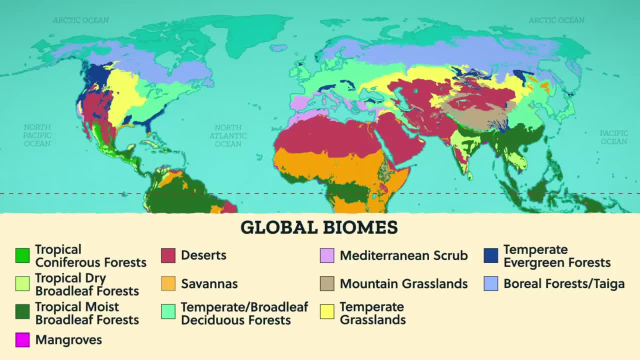 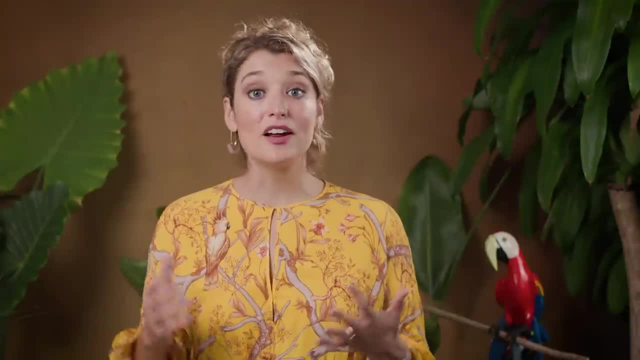 spruce, fir and larch trees At even higher latitudes. the decreasing temperatures give us the icy tundra biome with no trees and very little productivity. So the amount of energy flow through different ecosystems varies wildly, which limits which type of plants can thrive here. 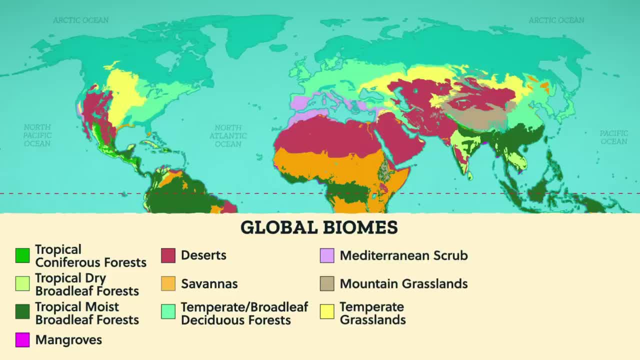 Up here in the middle of continents, there are temperate grassland biomes with rich soils that produce the tall grass of prairies and the short grass of steppe climates. Further north, where there are poorer soils and colder climates, we meet the boreal forest biomes, which have mainly evergreen pine. 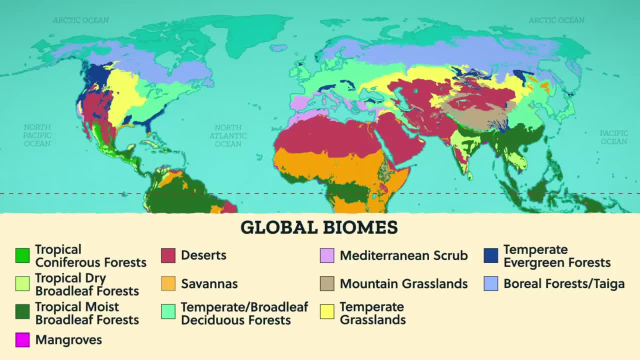 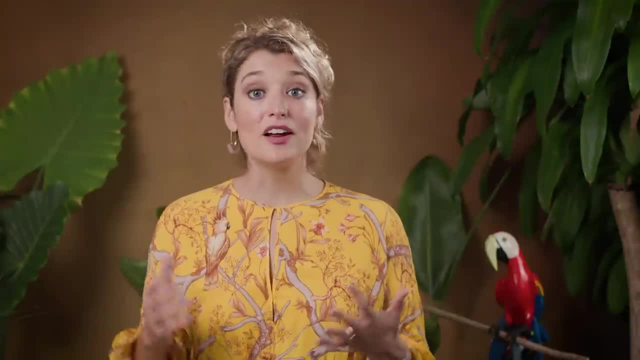 spruce, fir and larch trees At even higher latitudes. the decreasing temperatures give us the icy tundra biome with no trees and very little productivity. So the amount of energy flow through different ecosystems varies wildly, which limits which type of plants can thrive here. 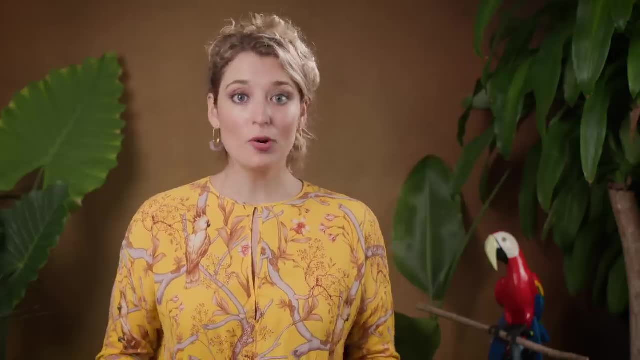 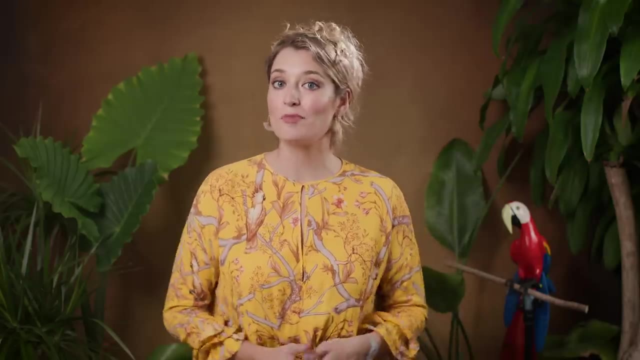 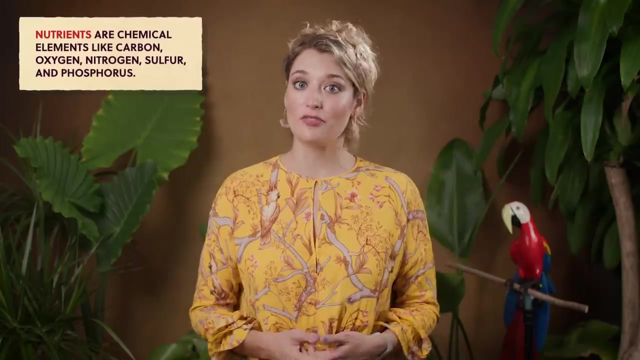 And because plants feed more consumers than any other food source. more plants means more biodiversity, or the number of different plants and animals in an ecosystem, And we can't talk about biodiversity without the other key component of all ecosystems: Nutrients. Nutrients are chemical elements like carbon, oxygen, nitrogen, sulfur and phosphorus. 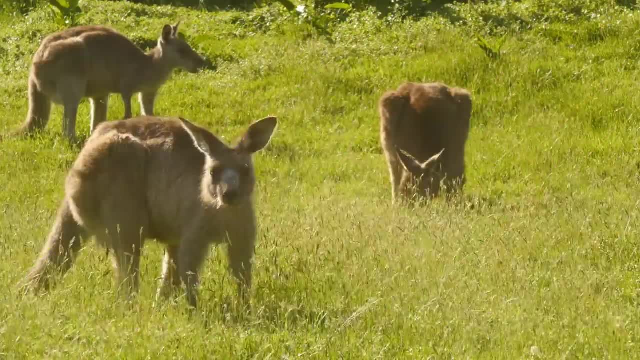 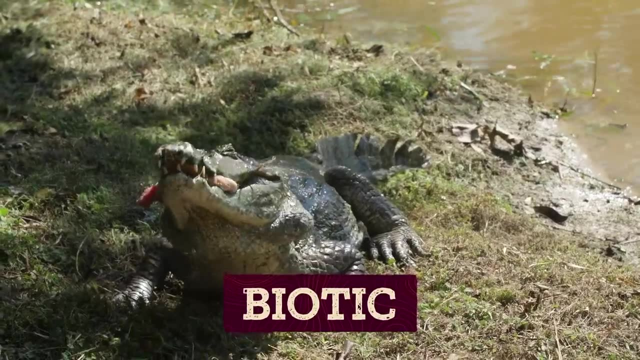 stored both in the living and non-living parts of an ecosystem, And we actually have technical terms for those too. The living things, like plants and animals and bacteria or their dead bodies are the biotic parts of an ecosystem, And the non-living things, like the soil, atmosphere and groundwater, are the abiotic parts. 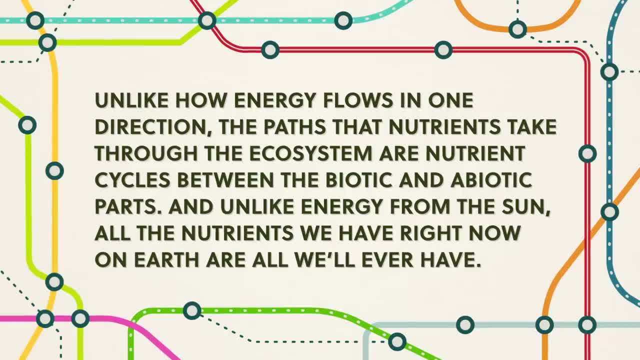 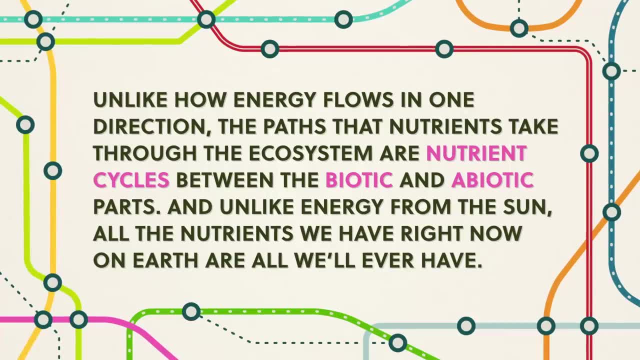 Unlike how energy flows in one direction, the paths that nutrients take through the ecosystem are nutrient cycles between the biotic and abiotic parts, And, unlike energy from the sun, all the nutrients we have right now on Earth are all we'll ever have. 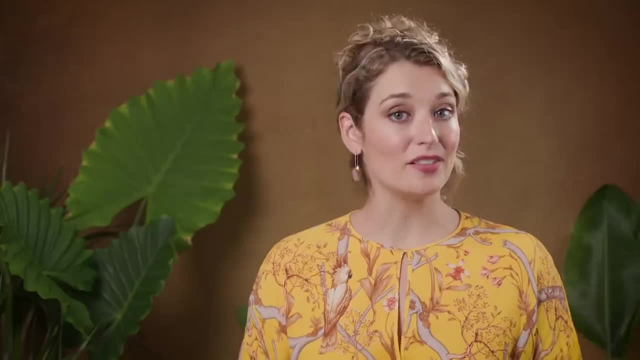 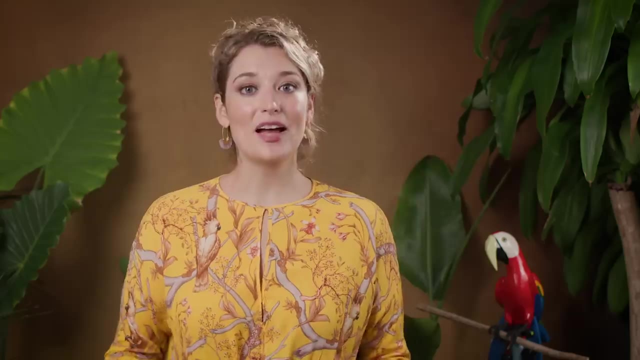 It's like how nitrogen moves from being a gas in the atmosphere to a solid in the soil, Instead of a one-way system like aliens dropping gift-wrapped boxes of nitrogen. the biotic parts of an ecosystem really help facilitate these nutrient cycles Like let's look at our fish tank ecosystem again. 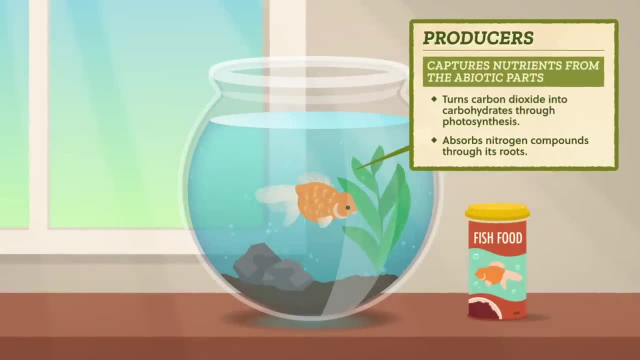 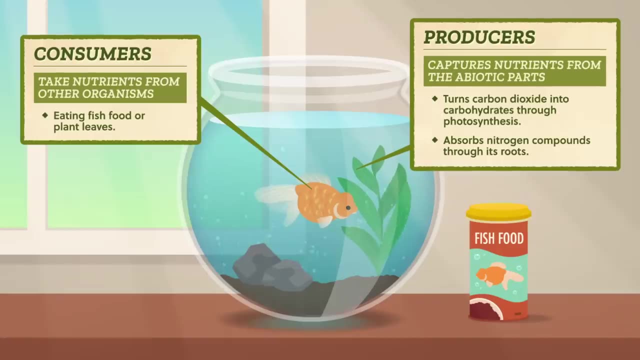 Producers, like our little plant, capture nutrients from the abiotic parts, turning carbon dioxide into carbohydrates through photosynthesis or absorbing nitrogen compounds through its roots. Consumers, like the fish, take nutrients from other organisms, munching on fish food or the plant's leaves. 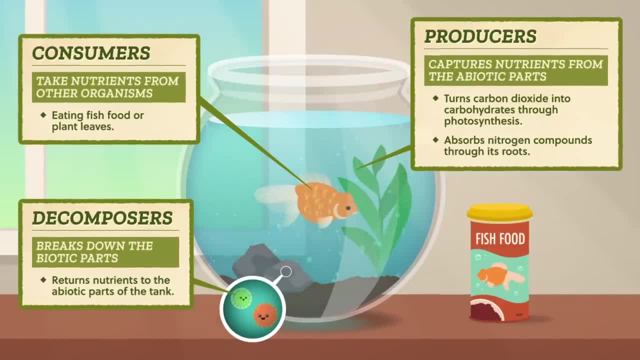 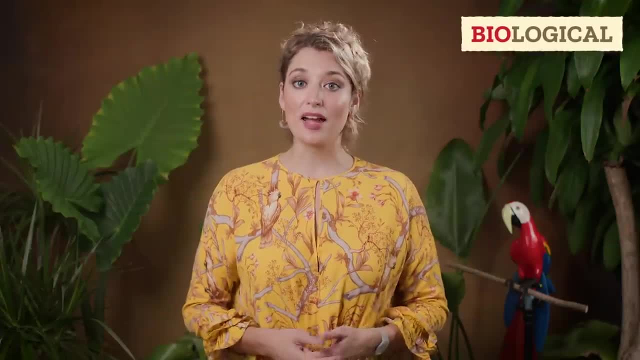 And decomposers break down dead plant leaves or our fish eventually, and return the nutrients, like nitrogen gas, to the abiotic parts of the tank. Ultimately, nutrient cycling through ecosystems depend on biological, geological and chemical processes operating within the atmosphere. 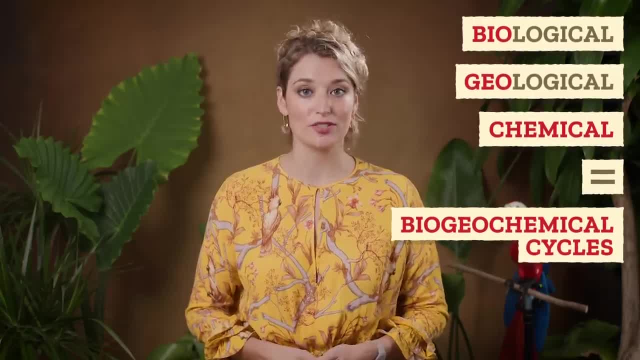 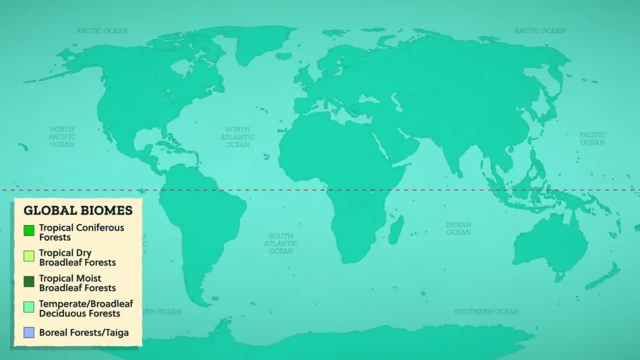 hydrosphere and lithosphere and make up Earth's biogeochemical cycles. We can compare nutrients across the Earth's biosphere, just like we compared net primary production across different latitudes and biomes, Like let's look at three biomes we met before. 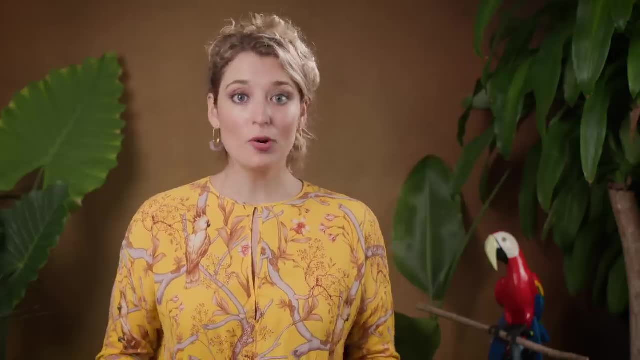 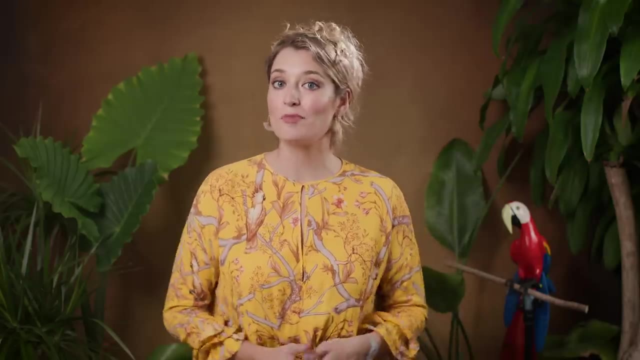 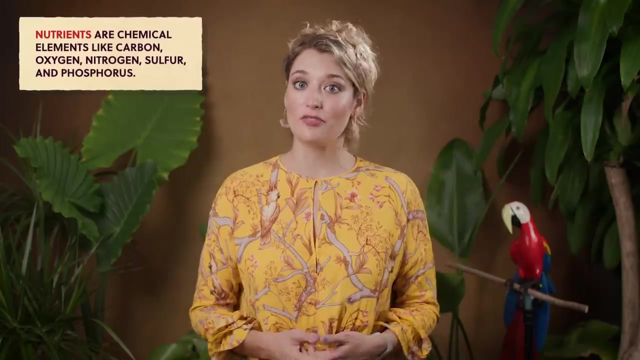 And because plants feed more consumers than any other food source. more plants means more biodiversity, or the number of different plants and animals in an ecosystem, And we can't talk about biodiversity without the other key component of all ecosystems: Nutrients. Nutrients are chemical elements like carbon, oxygen, nitrogen, sulfur and phosphorus. 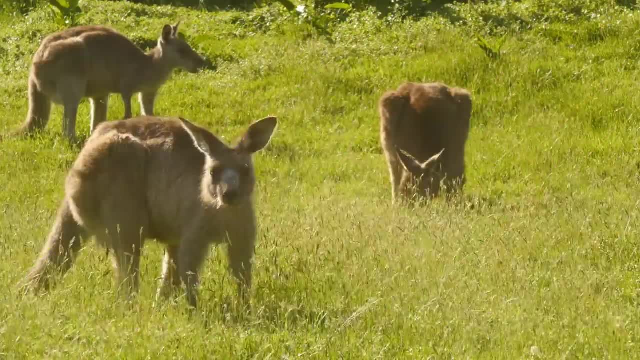 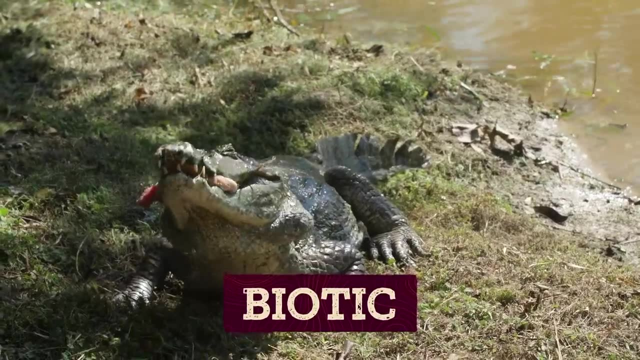 stored both in the living and non-living parts of an ecosystem, And we actually have technical terms for those too. The living things, like plants and animals and bacteria or their dead bodies are the biotic parts of an ecosystem, And the non-living things, like the soil, atmosphere and groundwater, are the abiotic parts. 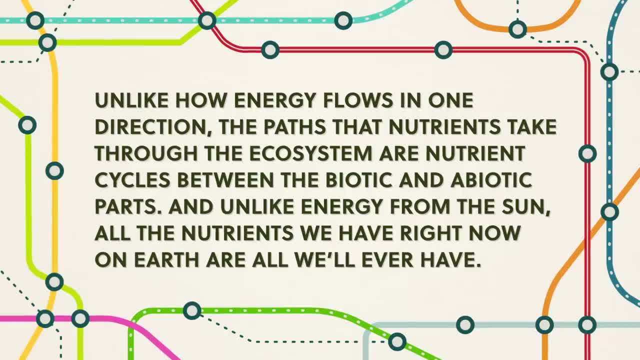 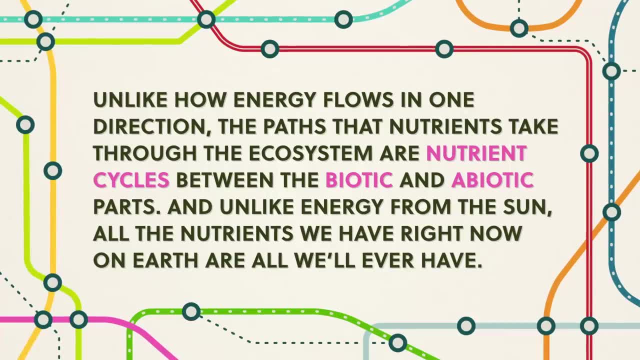 Unlike how energy flows in one direction, the paths that nutrients take through the ecosystem are nutrient cycles between the biotic and abiotic parts, And, unlike energy from the sun, all the nutrients we have right now on Earth are all we'll ever have. 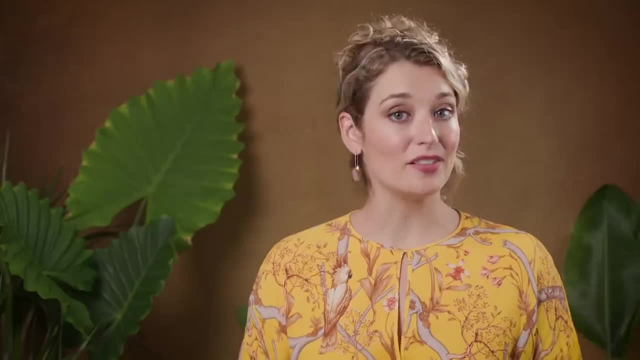 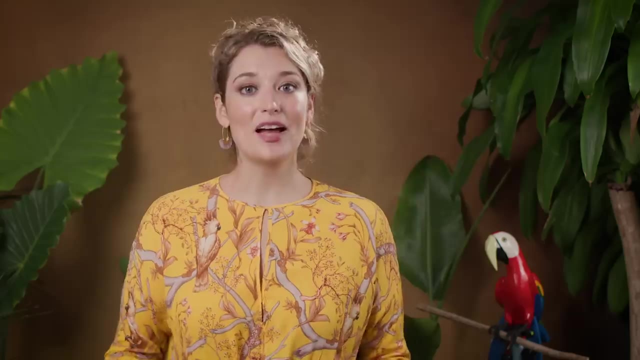 It's like how nitrogen moves from being a gas in the atmosphere to a solid in the soil, Instead of a one-way system like aliens dropping gift-wrapped boxes of nitrogen. the biotic parts of an ecosystem really help facilitate these nutrient cycles Like let's look at our fish tank ecosystem again. 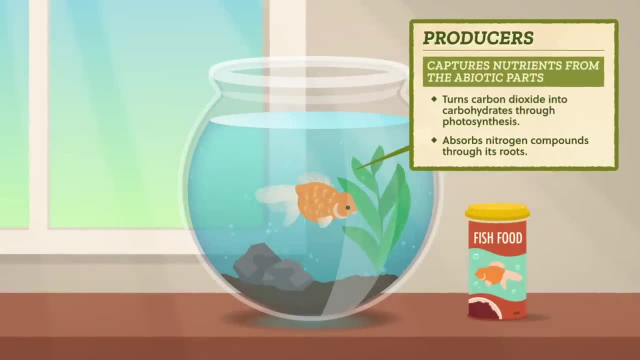 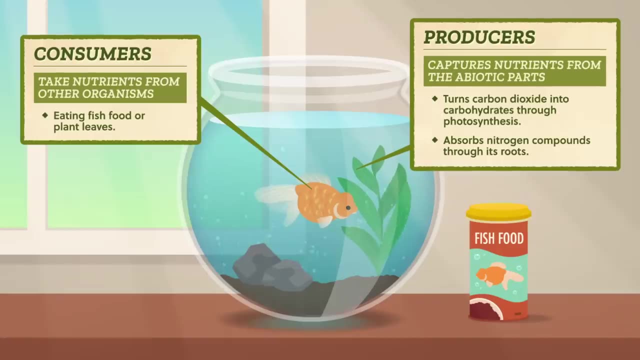 Producers, like our little plant, capture nutrients from the abiotic parts, turning carbon dioxide into carbohydrates through photosynthesis or absorbing nitrogen compounds through its roots. Consumers, like the fish, take nutrients from other organisms, munching on fish food or the plant's leaves. 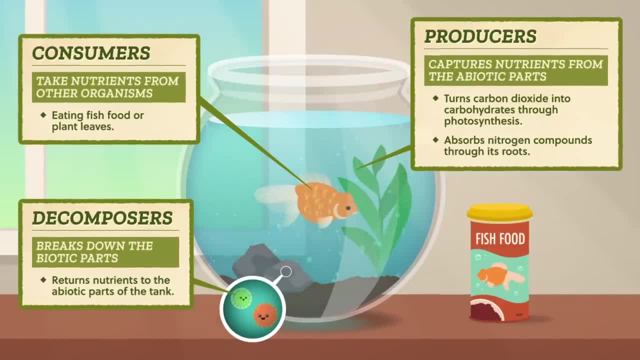 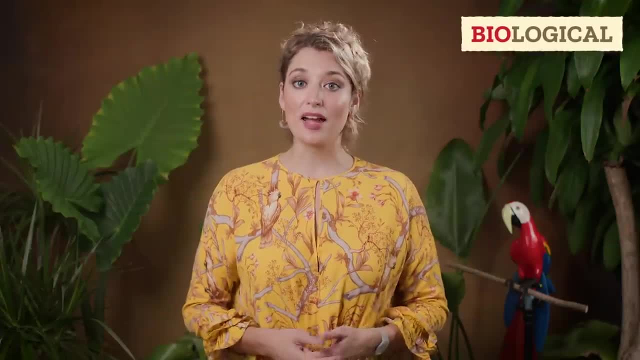 And decomposers break down dead plant leaves or our fish eventually, and return the nutrients, like nitrogen gas, to the abiotic parts of the tank. Ultimately, nutrient cycling through ecosystems depend on biological, geological and chemical processes operating within the atmosphere. 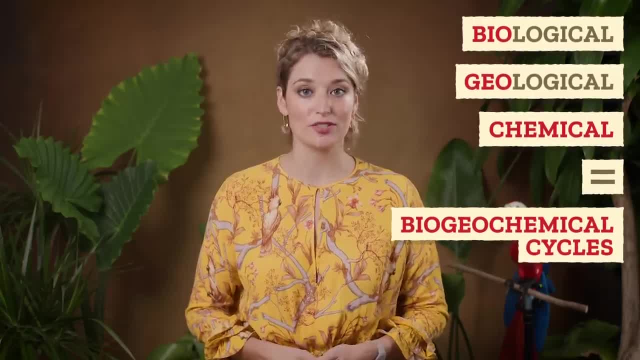 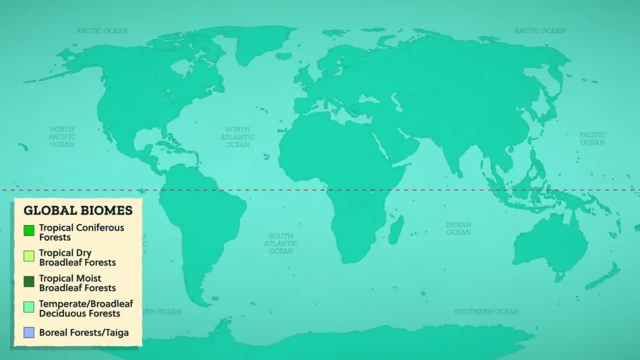 hydrosphere and lithosphere and make up Earth's biogeochemical cycles. We can compare nutrients across the Earth's biosphere, just like we compared net primary production across different latitudes and biomes, Like let's look at three biomes we met before. 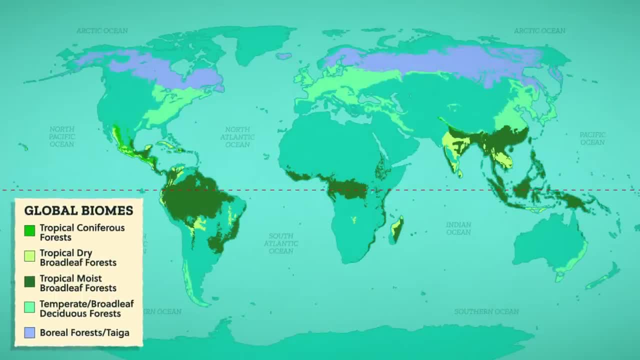 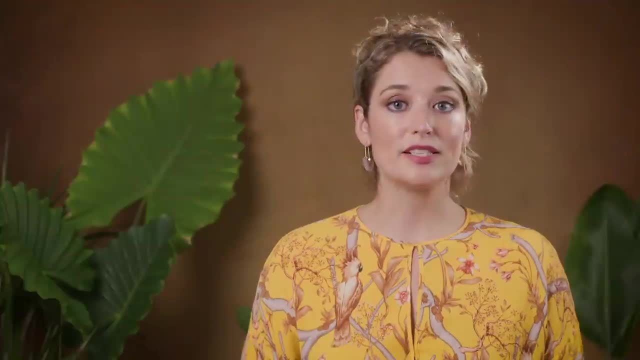 The tropical rainforest, deciduous forest and boreal forests. We know that there's less and less productivity as we move up in latitude, so there's less and less biomass and there's also less nutrients. Fewer nutrients isn't enough to make a big deal out of it. 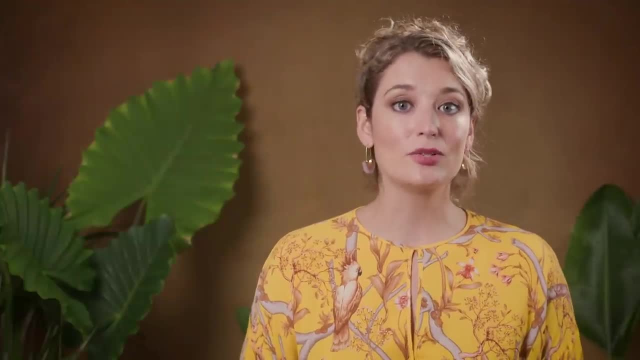 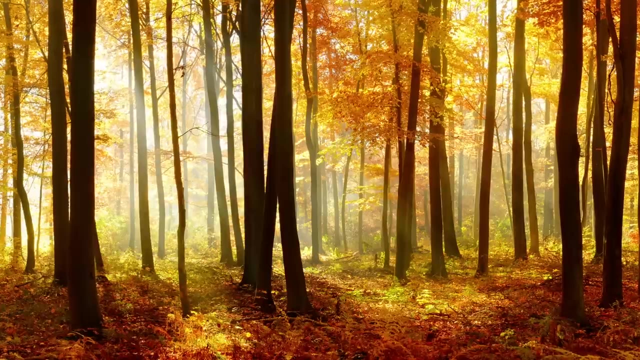 It isn't necessarily a death sentence for the trees, though. It just means that an ecosystem is structured differently. Like boreal, forests have a lot of nutrient-filled litter because the cold keeps material from decomposing, But deciduous forests have a lot of nutrient-rich soil because it's warm. 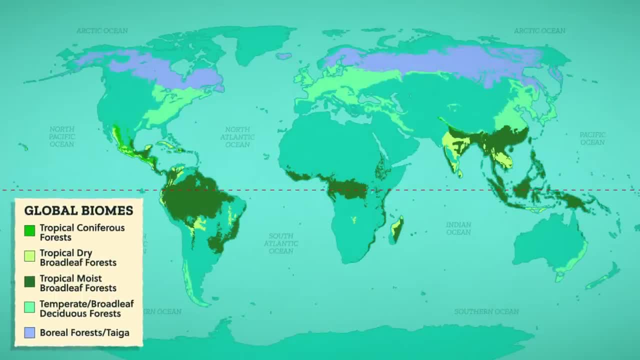 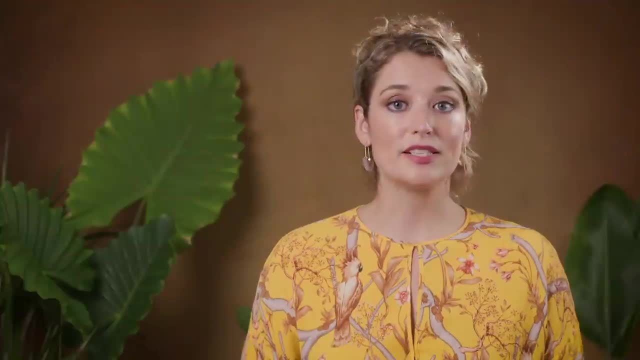 The tropical rainforest, deciduous forest and boreal forests. We know that there's less and less productivity as we move up in latitude, so there's less and less biomass and there's also less nutrients. Fewer nutrients isn't enough to make a big deal out of it. 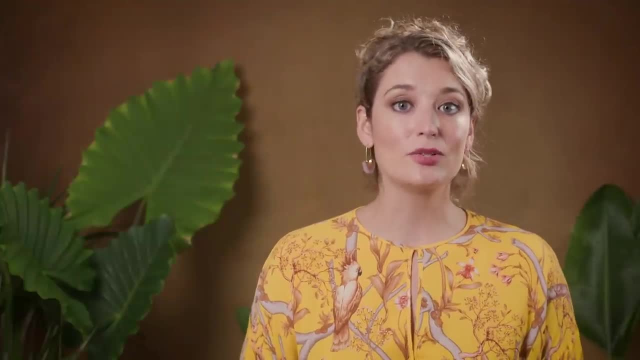 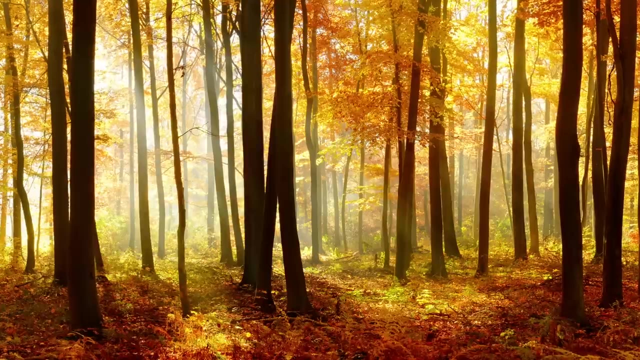 It isn't necessarily a death sentence for the trees, though. It just means that an ecosystem is structured differently. Like boreal, forests have a lot of nutrient-filled litter because the cold keeps material from decomposing, But deciduous forests have a lot of nutrient-rich soil because it's warm. 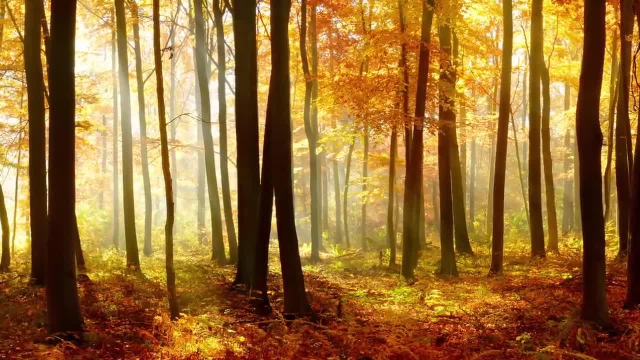 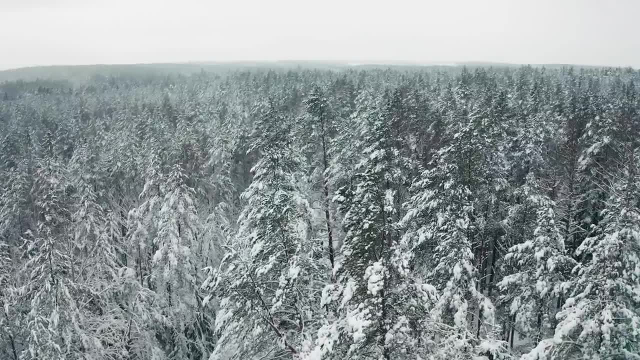 enough for material to decompose, but not warm enough for a lot of biomass to grow. So a tree that's adapted to life in a cold boreal forest might not make it in a tropical rainforest because of the different energy availability and nutrient stores. 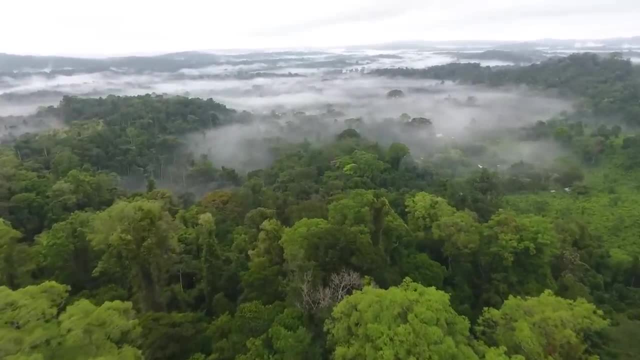 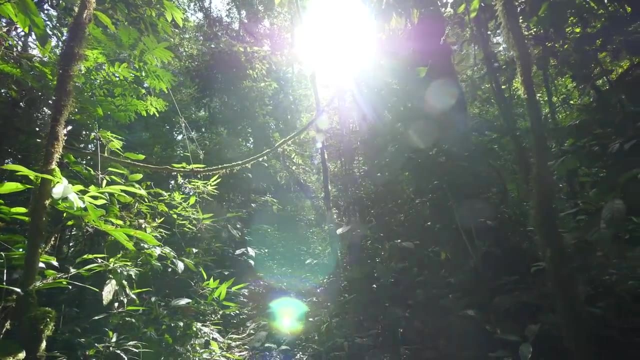 Let's consider the tropical rainforests, which are the most diverse biomes, with lush vegetation and a lot of biodiversity. But that decadence hides the fragile balance of all the complex energy flows and nutrient cycles. Let's go to the Thought Bubble. 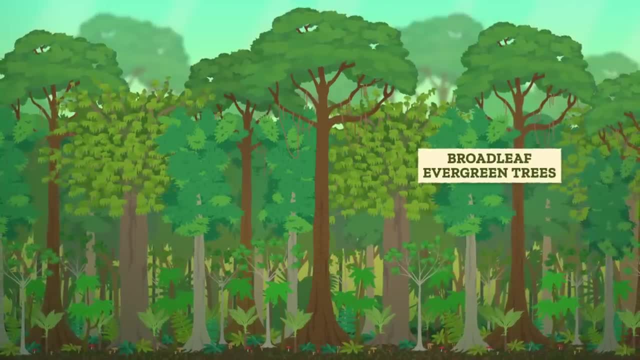 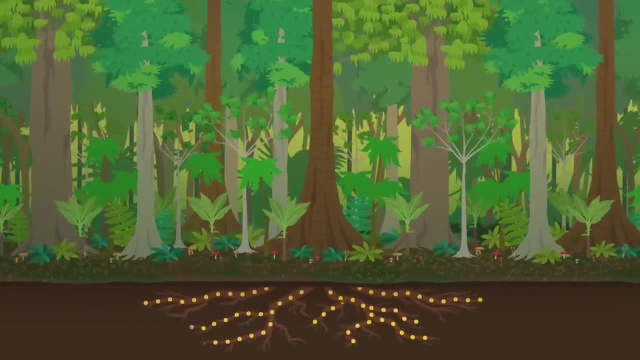 Within the tropical rainforests, broadleaf evergreen trees form a canopy at different heights, and little or no sunlight reaches the shady forest floor. These huge trees absorb most of the soil nutrients, which doesn't leave a lot for other organisms, And they have a shallow root system to grab as many of the minerals as possible from. 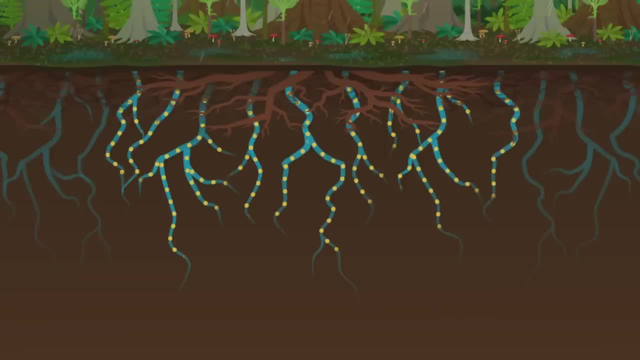 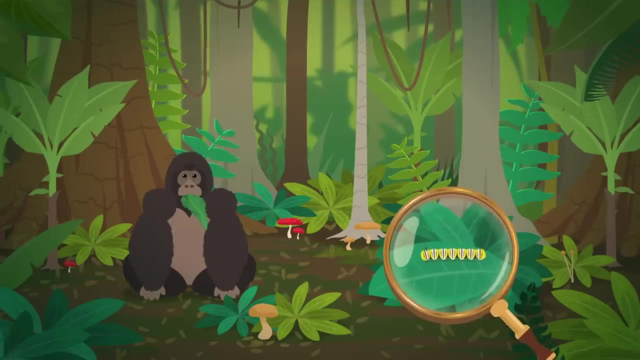 biogeochemical processes near the surface, And as the large amounts of rain filter down through the soil, the minerals that dissolve in water are leached away to inaccessible deeper levels. To survive, the rainforest has to rapidly cycle nutrients. The canopy trees are producers, along with understory plants that work together to keep 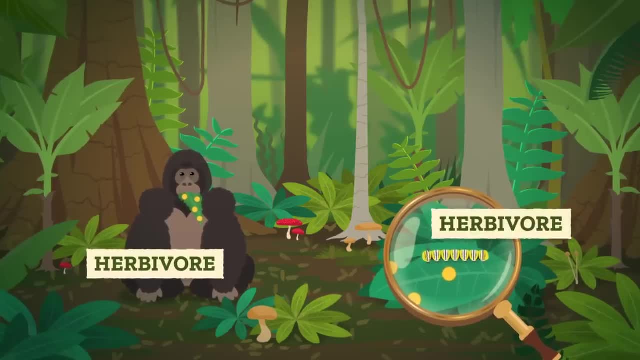 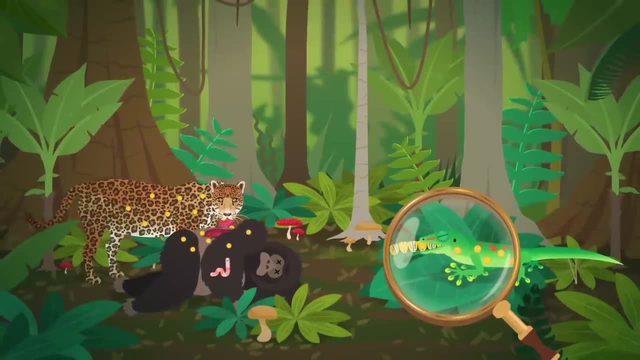 vital nutrients moving through the ecosystem. Herbivores like gorillas and caterpillars take in those nutrients and move them around through their excrement and by being eaten themselves, like by jaguars or geckos, And the warmth and humidity helps decomposers and their chemical reactions. so any dead plants or animals decay quickly Because nutrients get sucked from the soil so quickly. when those huge trees are cut down, the energy flows and nutrient cycles break. Those big producers aren't there to sustain consumers or shed leaves to recycle nutrients. 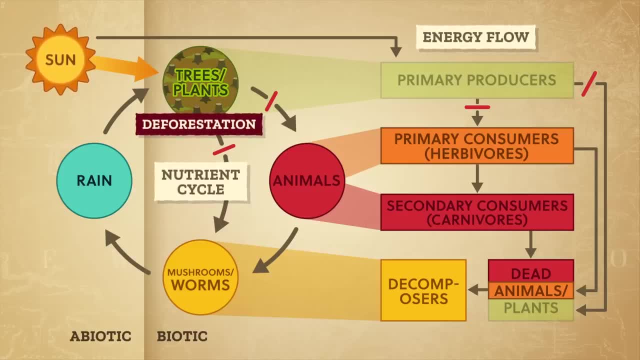 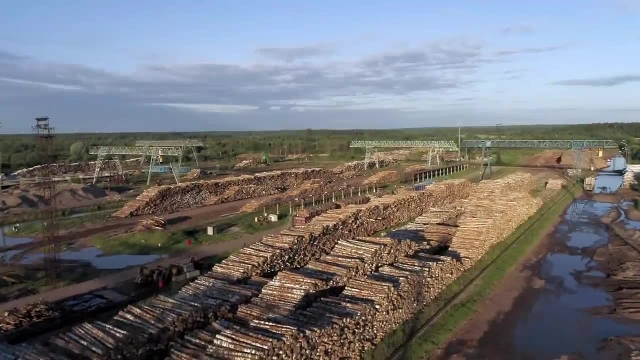 So deforestation or removing trees to use the land for something else can be especially destructive in tropical regions, if you don't consider the biogeochemical cycles. Thanks, Thought Bubble. We have negative associations with the word deforestation, for good reason. 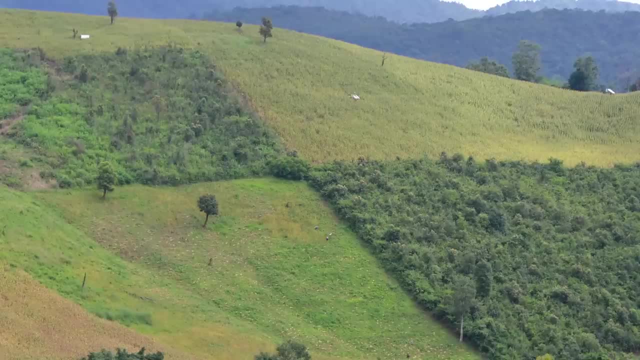 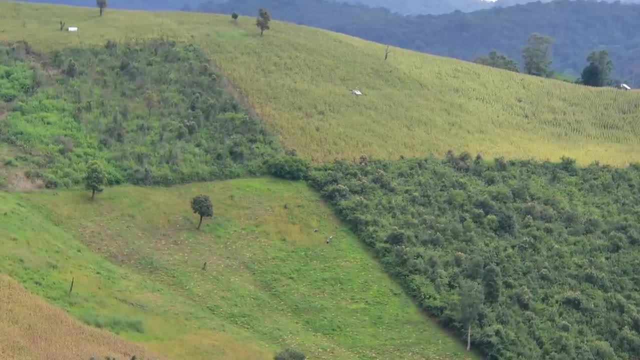 A lot of tree removal has caused immense damage to ecosystems, But indigenous communities have figured out a type of calculated clearing that allows them to work with the rapid nutrient recycling of tropical rainforest biomes. In parts of Asia, Africa and South America with dense tropical forests. 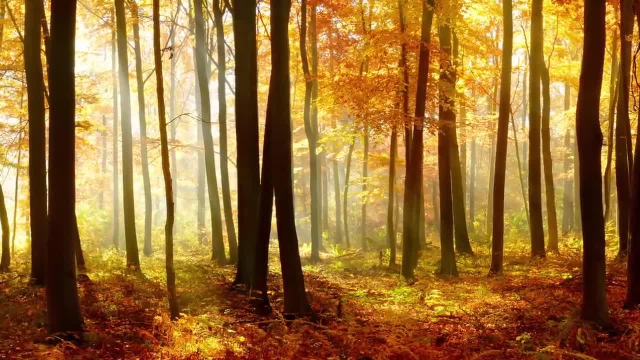 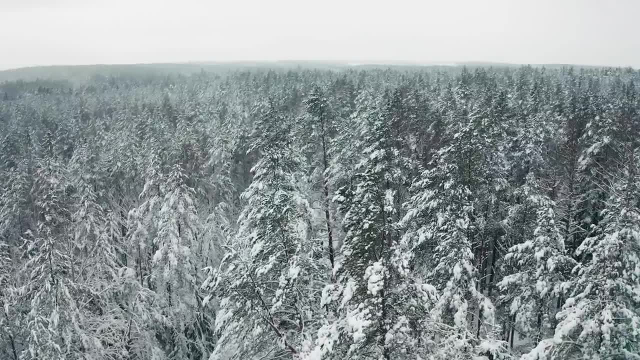 enough for material to decompose, but not warm enough for a lot of biomass to grow. So a tree that's adapted to life in a cold boreal forest might not make it in a tropical rainforest because of the different energy availability and nutrient stores. 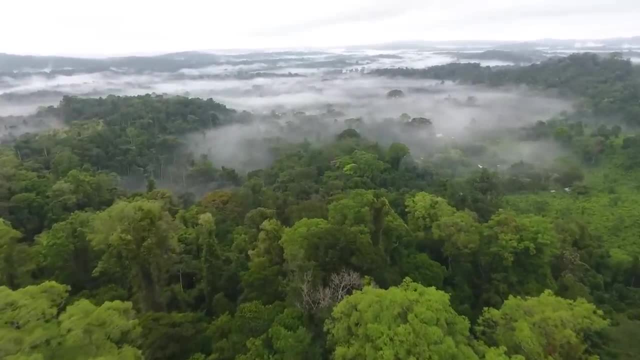 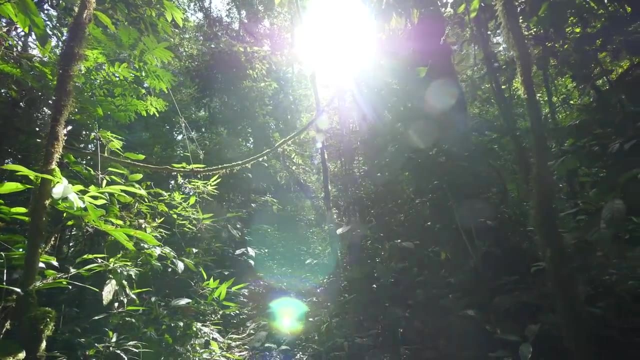 Let's consider the tropical rainforests, which are the most diverse biomes, with lush vegetation and a lot of biodiversity. But that decadence hides the fragile balance of all the complex energy flows and nutrient cycles. Let's go to the Thought Bubble. 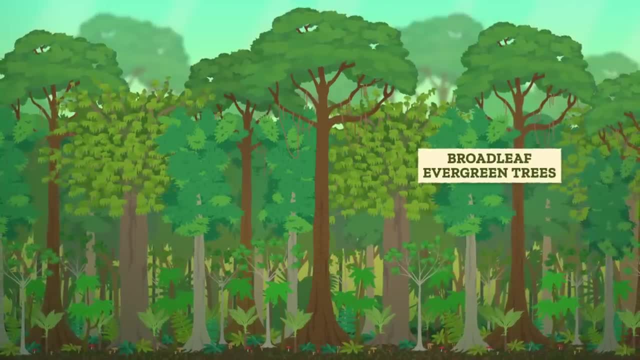 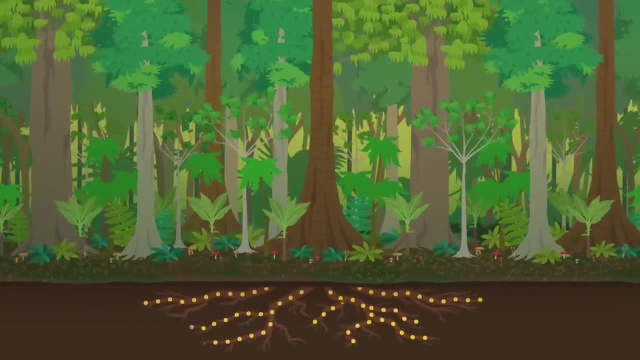 Within the tropical rainforests, broadleaf evergreen trees form a canopy at different heights, and little or no sunlight reaches the shady forest floor. These huge trees absorb most of the soil nutrients, which doesn't leave a lot for other organisms, And they have a shallow root system to grab as many of the minerals as possible from. 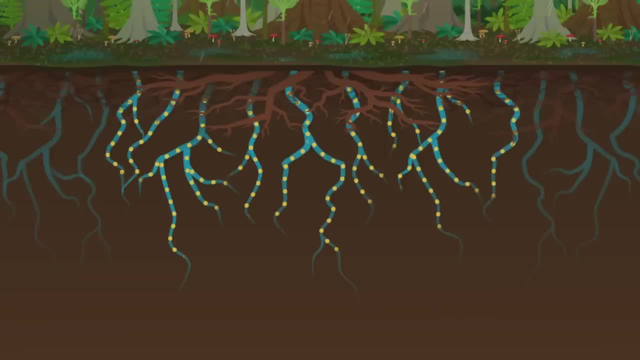 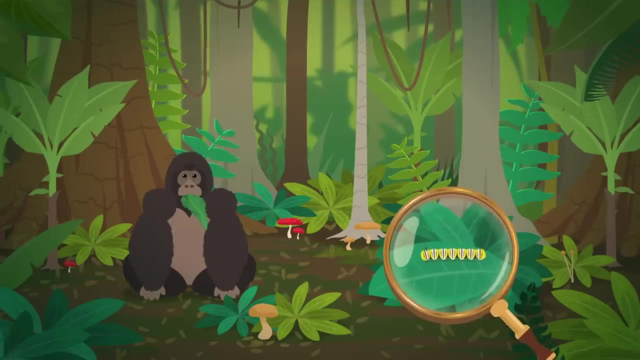 biogeochemical processes near the surface, And as the large amounts of rain filter down through the soil, the minerals that dissolve in water are leached away to inaccessible deeper levels. To survive, the rainforest has to rapidly cycle nutrients. The canopy trees are producers, along with understory plants that work together to keep 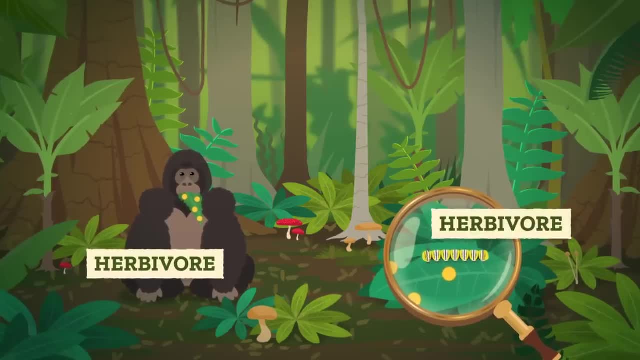 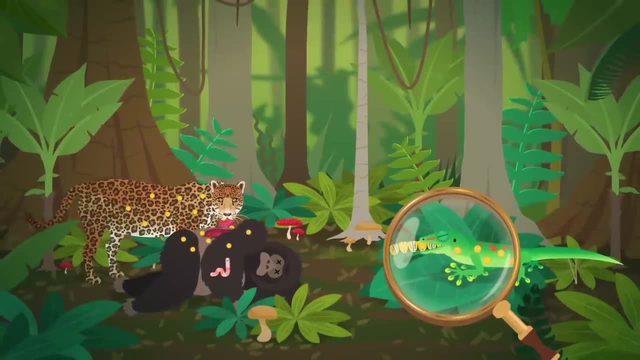 vital nutrients moving through the ecosystem. Herbivores like gorillas and caterpillars take in those nutrients and move them around through their excrement and by being eaten themselves, like by jaguars or geckos, And the warmth and humidity helps decomposers and their chemical reactions. so any dead plants or animals decay quickly Because nutrients get sucked from the soil so quickly. when those huge trees are cut down, the energy flows and nutrient cycles break. Those big producers aren't there to sustain consumers or shed leaves to recycle nutrients. 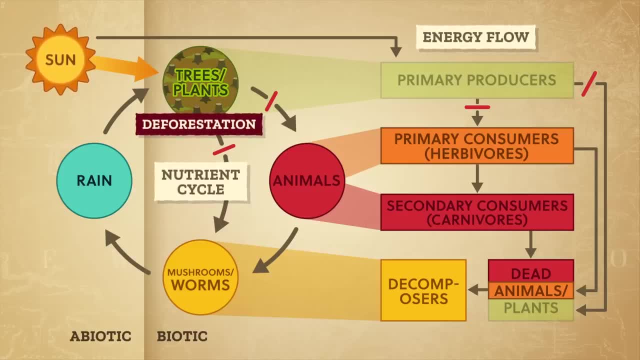 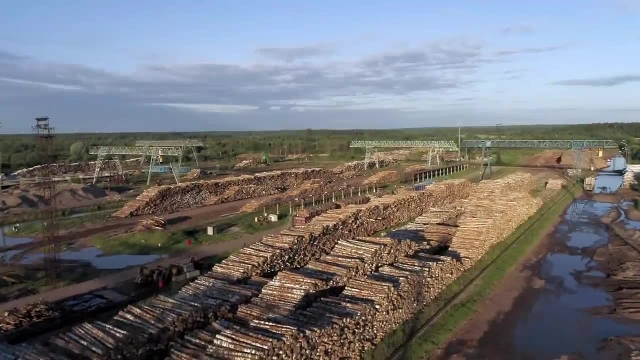 So deforestation or removing trees to use the land for something else can be especially destructive in tropical regions, if you don't consider the biogeochemical cycles. Thanks, Thought Bubble. We have negative associations with the word deforestation, for good reason. 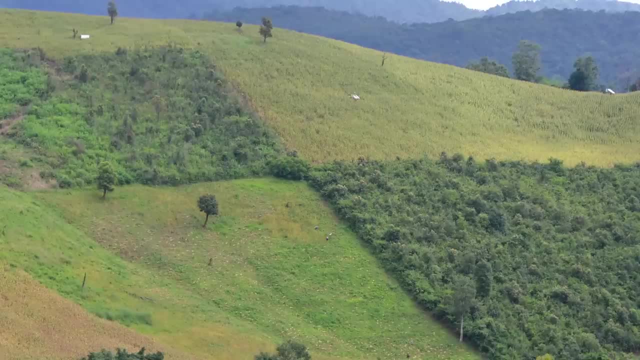 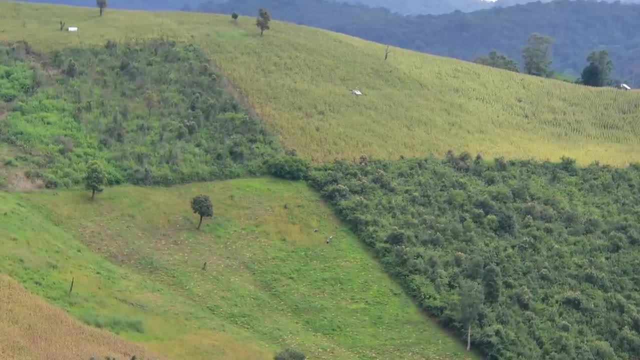 A lot of tree removal has caused immense damage to ecosystems, But indigenous communities have figured out a type of calculated clearing that allows them to work with the rapid nutrient recycling of tropical rainforest biomes. In parts of Asia, Africa and South America with dense tropical forests. 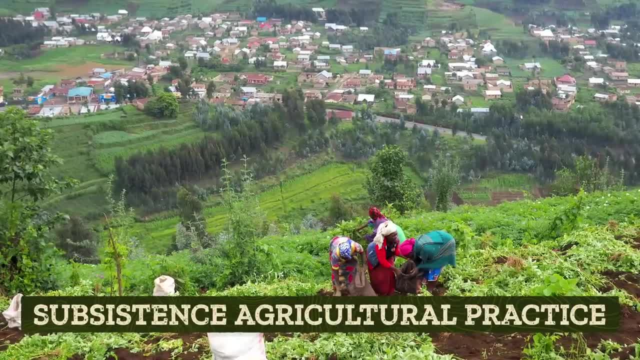 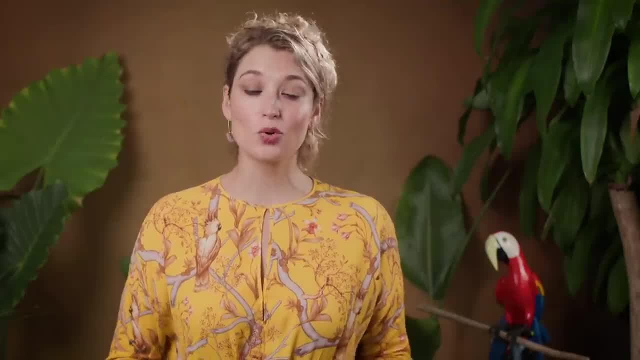 many farmers have to rely on a kind of subsistence agricultural practice, which means they only grow enough food for their families. Staples like rice are grown in Southeast Asia, maize and cassava in South America and sorghum in Africa. Yams, sugarcane, plantains and vegetables are also planted to supplement staples and 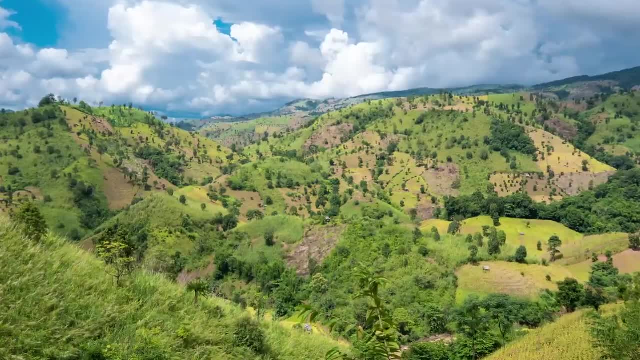 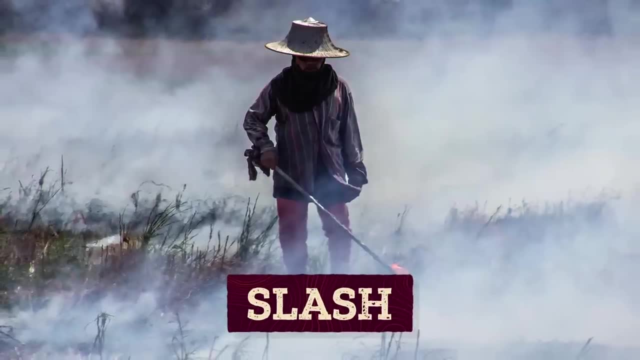 to provide fuel and fodder for animals. This practice goes by many names like swidden, shifting cultivation and slash-and-burn agriculture. The farmers begin by cutting small areas of tropical forest into slash or cut vegetation that's then dried and burned. The ash gets mixed with the poor soil to provide needed minerals and nutrients, basically using all the good stuff stored up in the vegetation biomass to help new crop plants grow. Of course, these crop plants use minerals and nutrients from the soil as they grow. 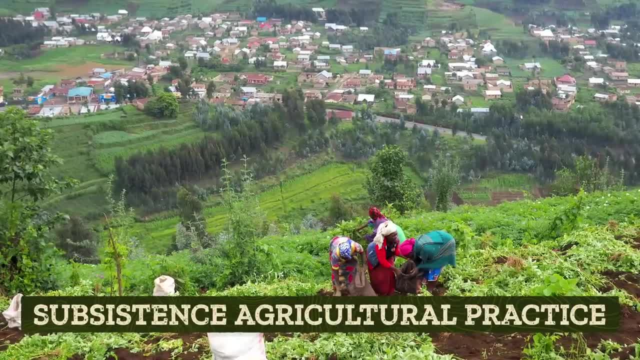 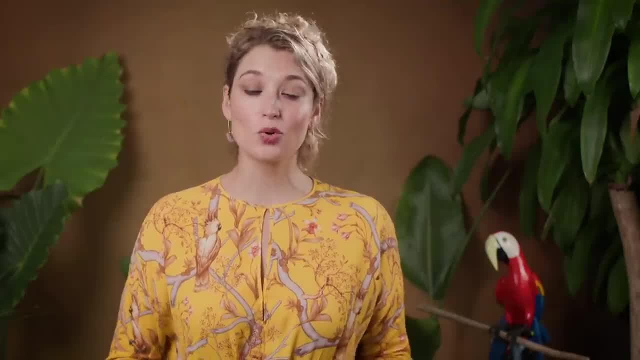 many farmers have to rely on a kind of subsistence agricultural practice, which means they only grow enough food for their families. Staples like rice are grown in Southeast Asia, maize and cassava in South America and sorghum in Africa. Yams, sugarcane, plantains and vegetables are also planted to supplement staples and 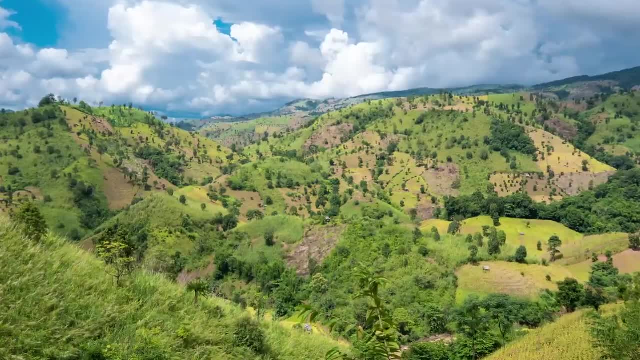 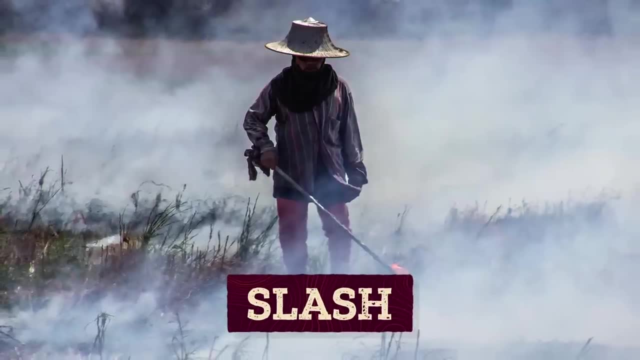 to provide fuel and fodder for animals. This practice goes by many names like swidden, shifting cultivation and slash-and-burn agriculture. The farmers begin by cutting small areas of tropical forest into slash or cut vegetation that's then dried and burned. The ash gets mixed with the poor soil to provide needed minerals and nutrients, basically using all the good stuff stored up in the vegetation biomass to help new crop plants grow. Of course, these crop plants use minerals and nutrients from the soil as they grow. 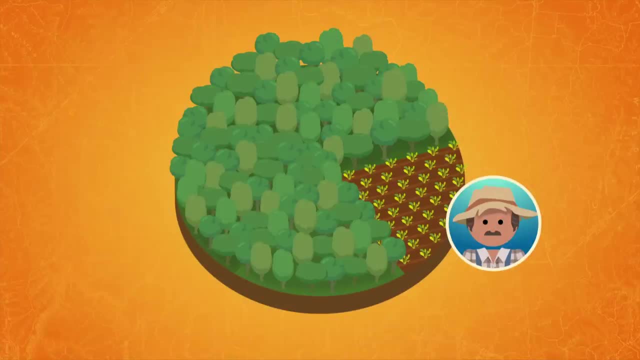 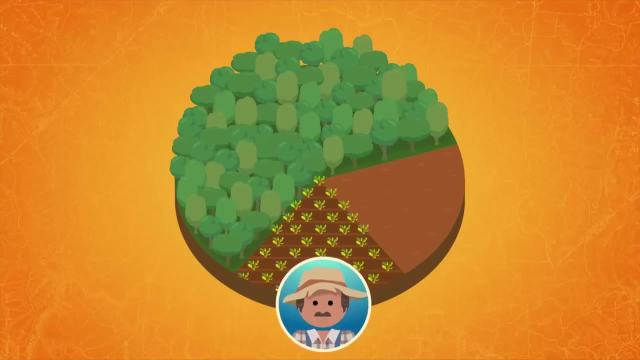 and we eat them to get those minerals and nutrients in our bodies. So after a few years and before the soil is completely exhausted, the farmers move on to another part of the land and repeat the clearing, burning and planting process. The previous plot is left up here, but I'm not going to go into all the details. 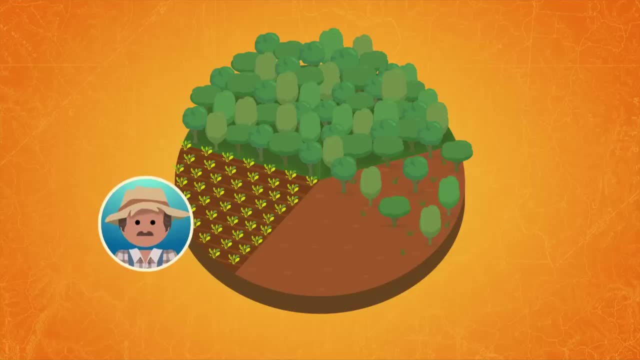 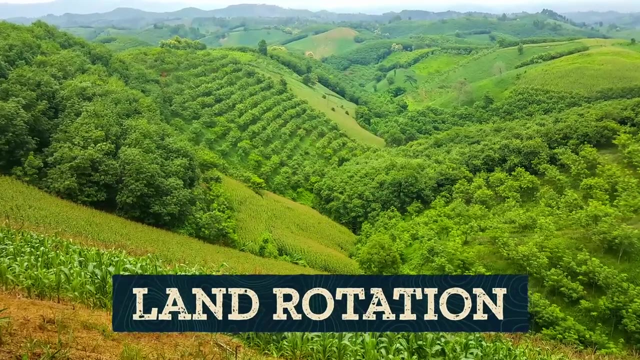 The soil is left unplanted and eventually the forest will naturally expand to start using that soil as part of its carefully balanced nutrient cycling. This land rotation is a key part of why humans have been able to keep farming like this for thousands of years. 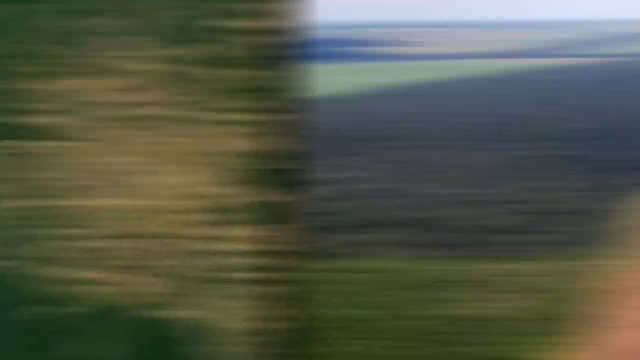 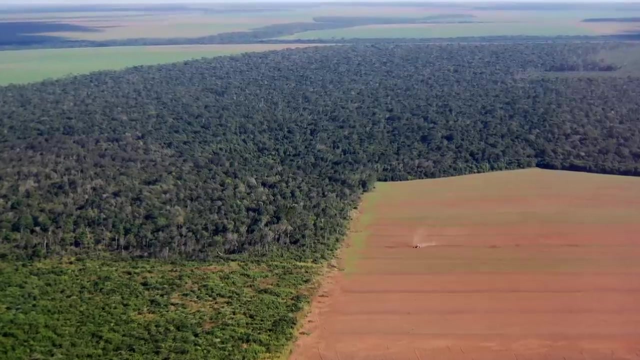 But when widespread clearcutting happens, ecosystems can collapse. For example, we've seen this destruction in the Amazon. when rice, soy and corn have been commercially cultivated and sold in domestic and international markets, The soil is exhausted after 3-5 years, so crops can't really grow anymore. 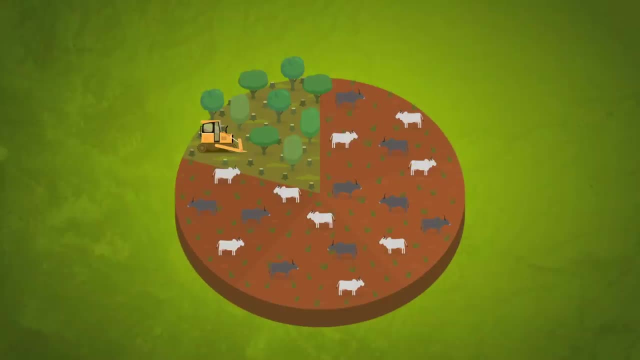 and then large cattle operations move in. As cattle feed and trample the ground, the soils are exposed to plenty of UV radiation. from sunlight, as well as cycles of wetting and drying from precipitation, The soils become a brick-like substance called laterite, which isn't great for growing. 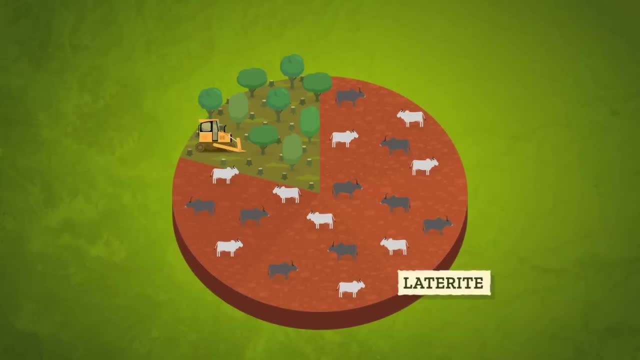 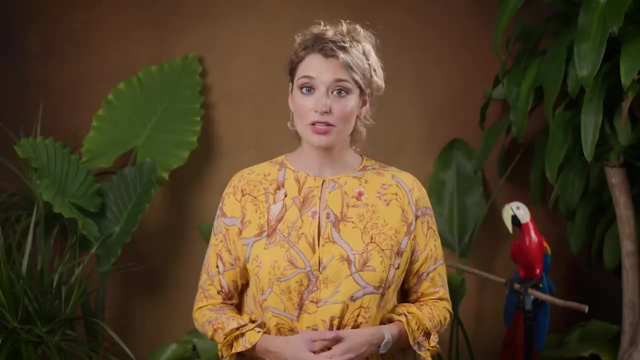 so the once lively rainforest basically becomes hard, barren and lifeless. Tropical rainforests cover 6% of Earth's landmass but contain 50% of the world's species, many of which haven't been described by science and are critical to the world's biodiversity. 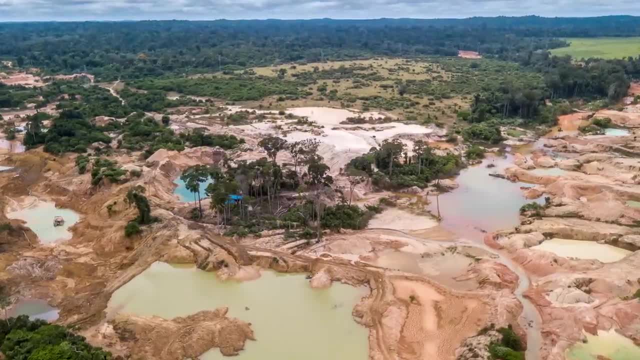 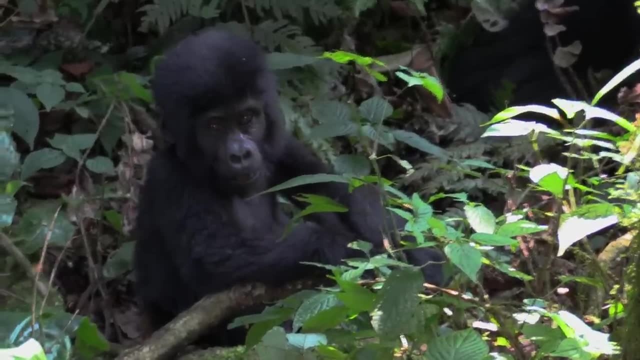 But since the 1980s, one fifth of the Amazon has been deforested. as we build more towns, roads, dams, farms and mines Across the Atlantic, deforestation in Ituri, in the Congo Basin, the world's second largest expanse of equatorial rainforest, is endangering the 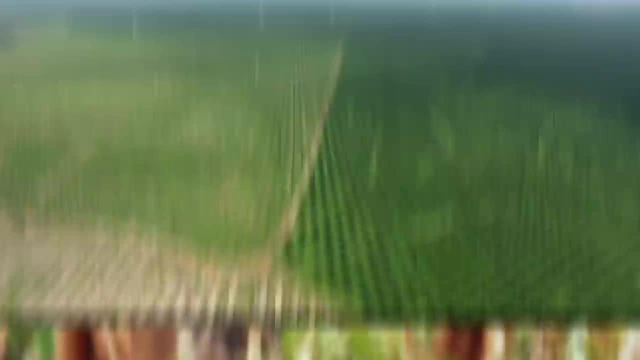 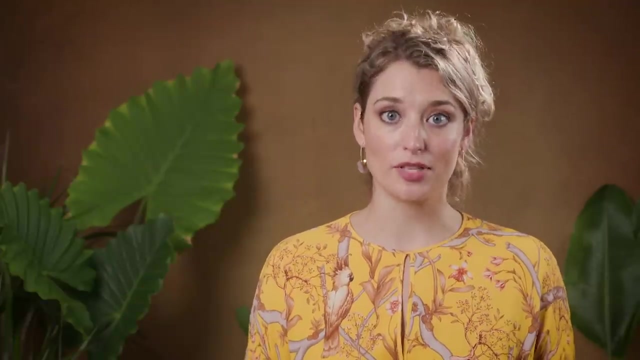 mountain gorilla, And in Southeast Asia, clearcutting for palm oil plantations endanger orangutans, Sumatran tigers and Sumatran elephants. When humans disturb the biosphere, we alter how energy flows and how nutrients cycle. 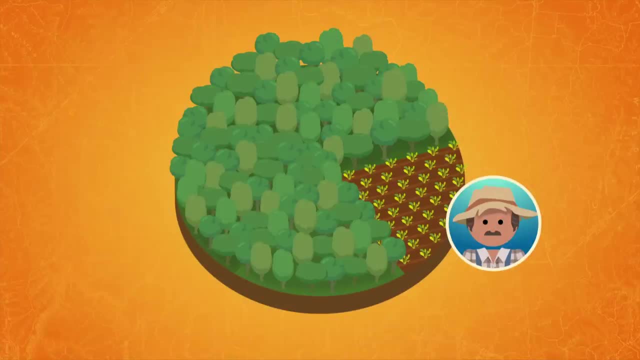 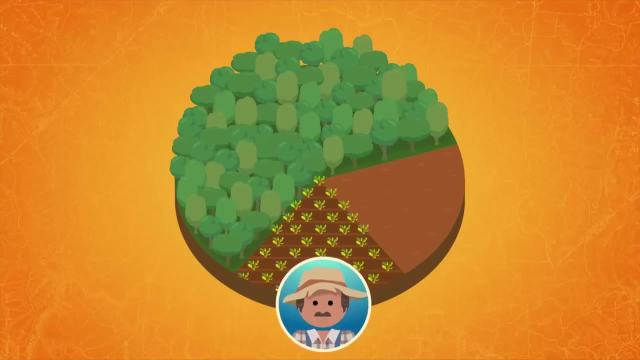 and we eat them to get those minerals and nutrients in our bodies. So after a few years and before the soil is completely exhausted, the farmers move on to another part of the land and repeat the clearing, burning and planting process. The previous plot is left up here, but I'm not going to go into all the details. 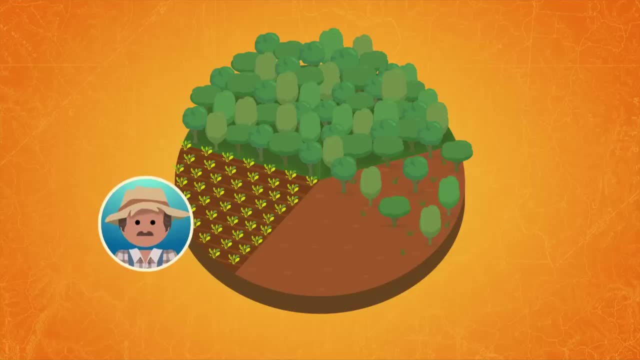 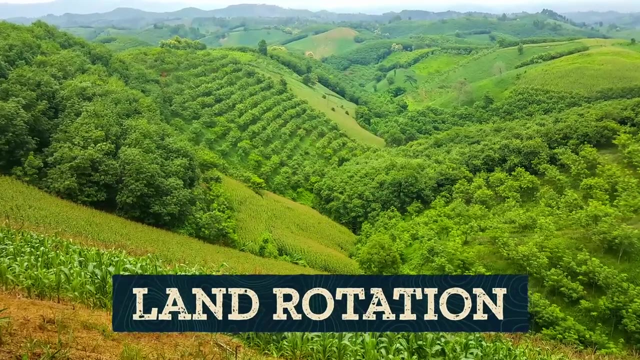 The soil is left unplanted and eventually the forest will naturally expand to start using that soil as part of its carefully balanced nutrient cycling. This land rotation is a key part of why humans have been able to keep farming like this for thousands of years. 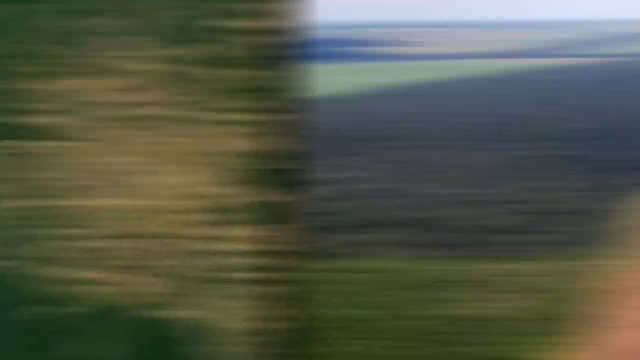 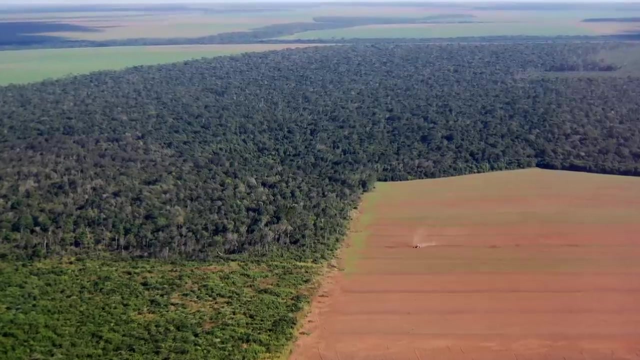 But when widespread clearcutting happens, ecosystems can collapse. For example, we've seen this destruction in the Amazon. when rice, soy and corn have been commercially cultivated and sold in domestic and international markets, The soil is exhausted after 3-5 years, so crops can't really grow anymore. 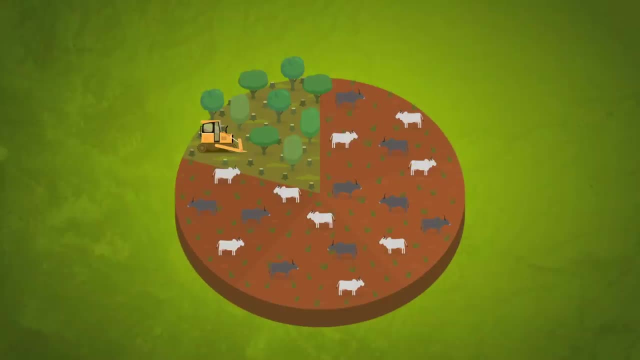 and then large cattle operations move in. As cattle feed and trample the ground, the soils are exposed to plenty of UV radiation. from sunlight, as well as cycles of wetting and drying from precipitation, The soils become a brick-like substance called laterite, which isn't great for growing. 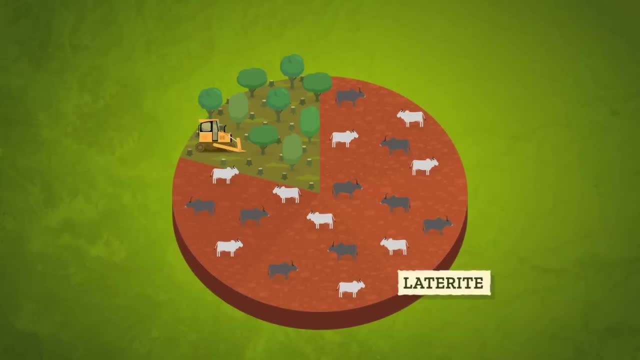 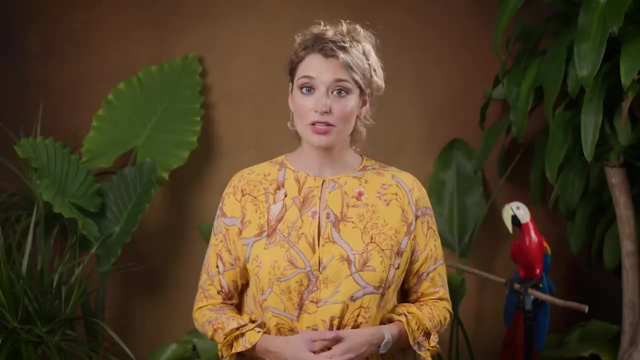 so the once lively rainforest basically becomes hard, barren and lifeless. Tropical rainforests cover 6% of Earth's landmass but contain 50% of the world's species, many of which haven't been described by science and are critical to the world's biodiversity. 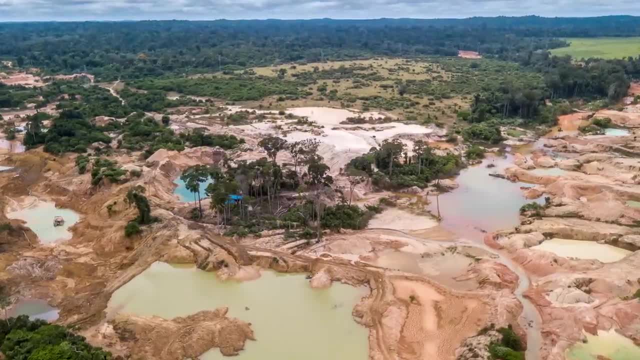 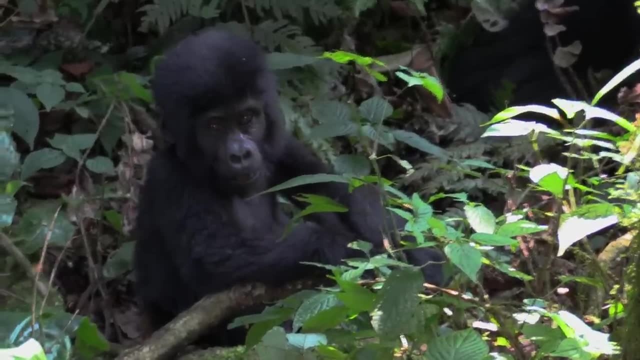 But since the 1980s, one fifth of the Amazon has been deforested. as we build more towns, roads, dams, farms and mines Across the Atlantic, deforestation in Ituri, in the Congo Basin, the world's second largest expanse of equatorial rainforest, is endangering the 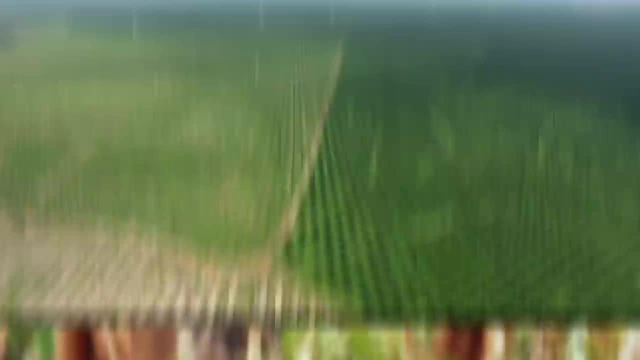 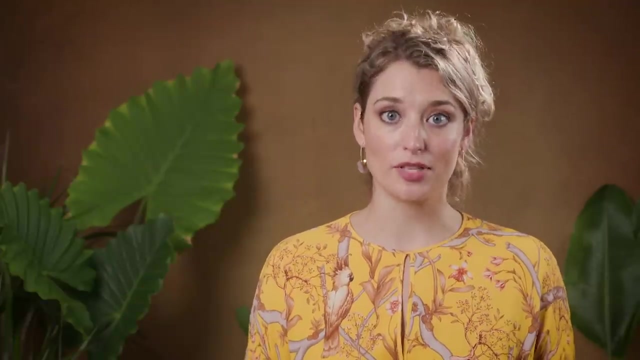 mountain gorilla, And in Southeast Asia, clearcutting for palm oil plantations endanger orangutans, Sumatran tigers and Sumatran elephants. When humans disturb the biosphere, we alter how energy flows and how nutrients cycle. 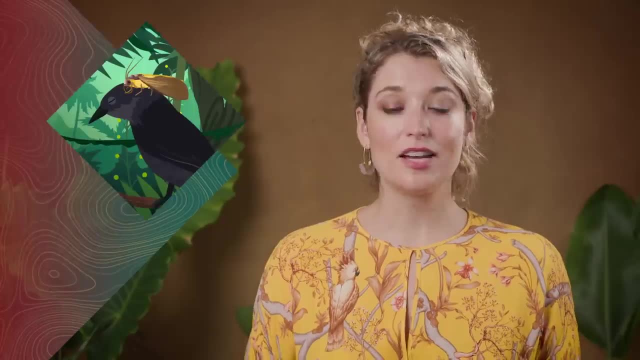 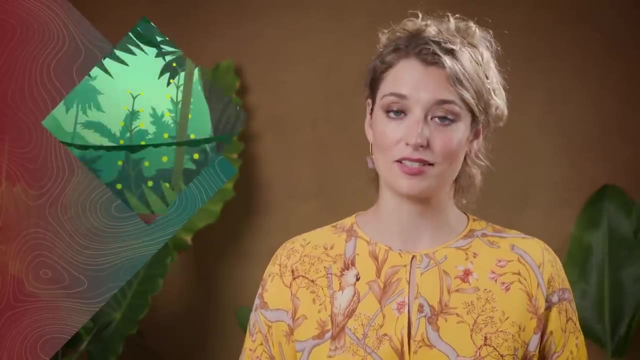 which can throw off entire ecosystems. in unexpected ways, And if we're not careful, that moth that drinks the tears of sleeping birds or plenty of other remarkable living organisms may no longer exist. But just like we can be good stewards of our little fish tank. 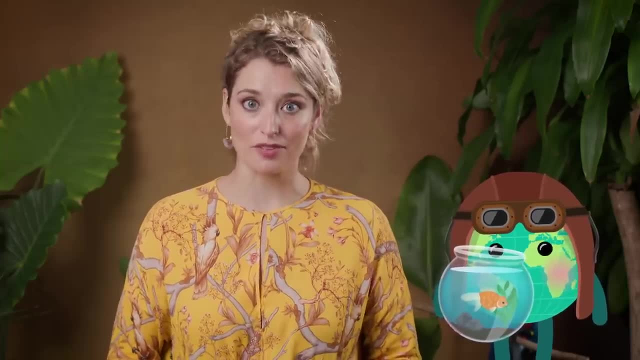 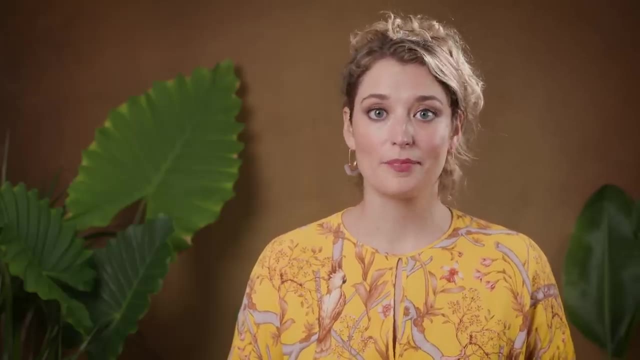 we can take care of the world around us and the much bigger ecosystems we're a part of. Learning where our food comes from and how it's produced is a good first step, like by supporting farmers who try to grow food sustainably, And we'll keep talking about our role in ecosystems, energy and food.